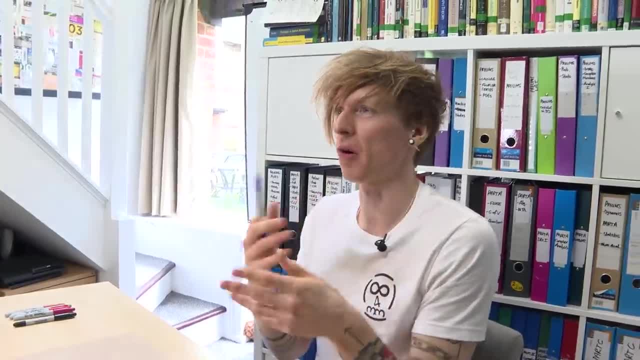 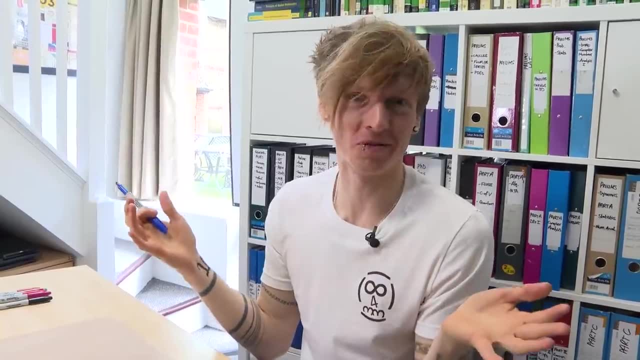 as mathematicians we wanted to be able to solve all possible quadratic equations. So we said: let's call the root of minus 1, i, and now we have a solution to any possible quadratic equation by the quadratic formula. But the best way to think about these is to draw a. 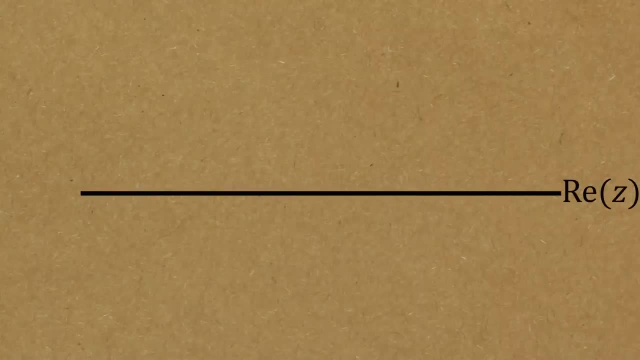 graph We have: the x-axis is the real part of z, the y-axis is the imaginary part of z, and then I can represent my complex number as actually a point in 2D space with coordinates x, y. So I go x across. let's say that's here. 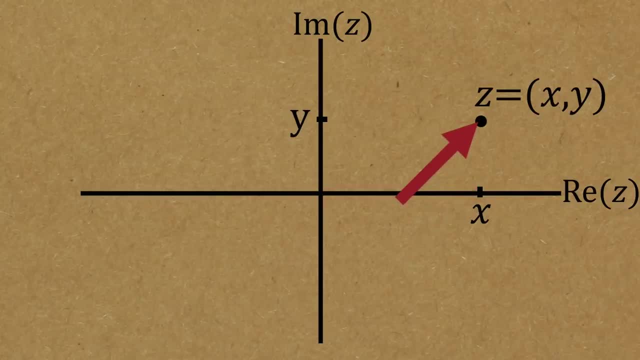 and then I can represent my complex number as actually a point in 2D space with coordinates x, y, And then I can represent my complex number as actually a point in 2D space with coordinates x, y, Then I go y up. so that's going to be about there. So this position, z, is equal to position. 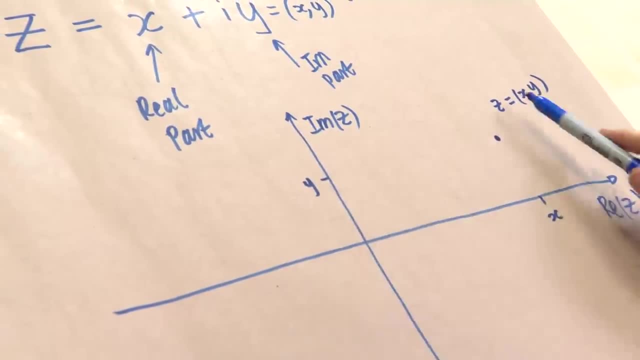 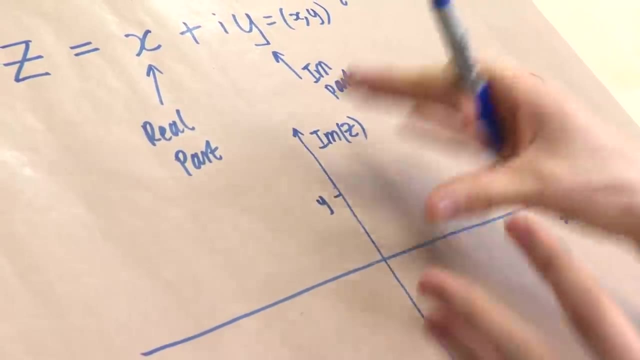 x, y in my 2D space, And this actually uniquely defines my complex number, because if I say to you, let's go x across here and y up, there's no other point that satisfies that particular property or that definition. Now, that's one way of representing a complex number. 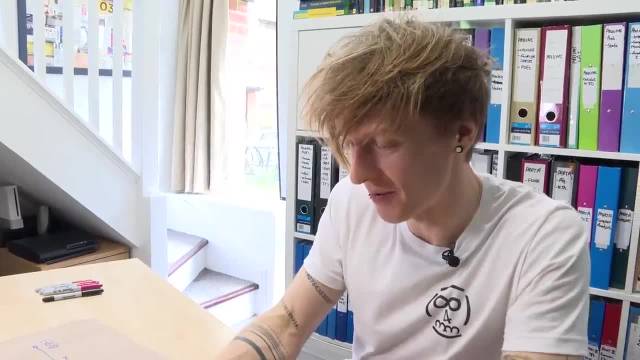 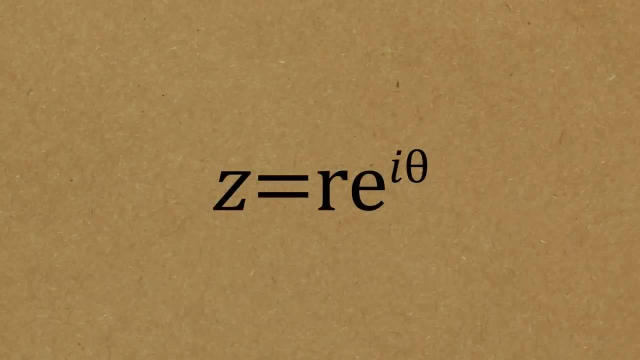 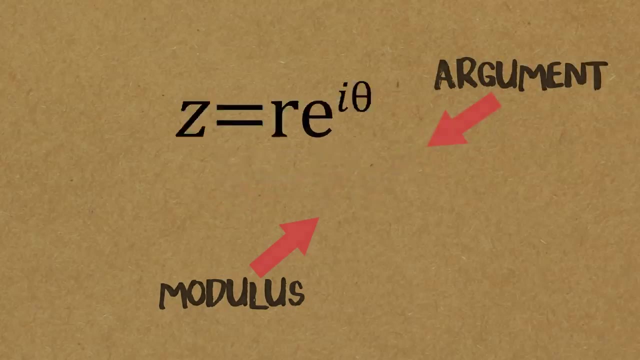 And now there's another way, which is the polar form. So for that one we have, z is equal to r, e to the i, theta, And here r we call this the modulus of z and theta represents the argument of z. Now these are just fancy words, which basically the modulus means the distance. 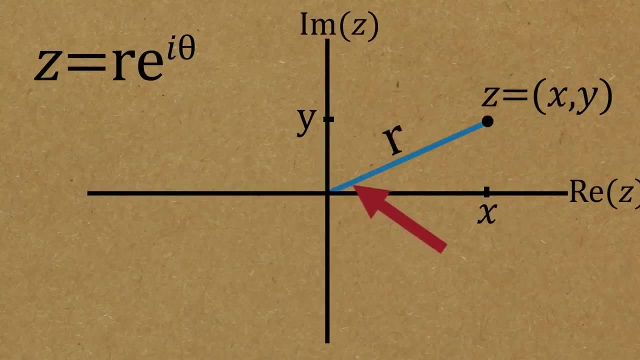 from the origin to our complex number. So if I draw a straight line which is the shortest distance between two points, this distance is r and that's this modulus of z which goes here. And then theta is an angle. and the angle is important because if I just told, 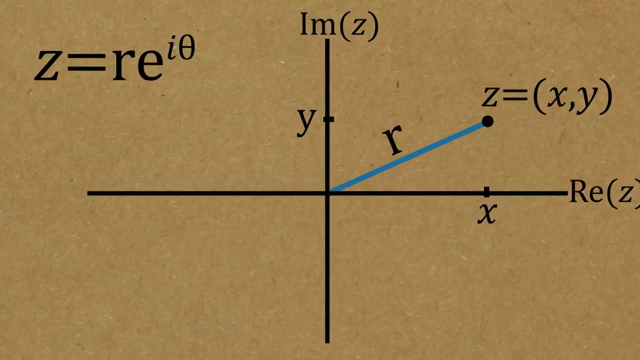 you we're at a distance r from the origin, then I could be here, but maybe I'm up here. This is also a distance r from the origin and in fact you're going to get a circle. All of these points will be a distance r from the origin. 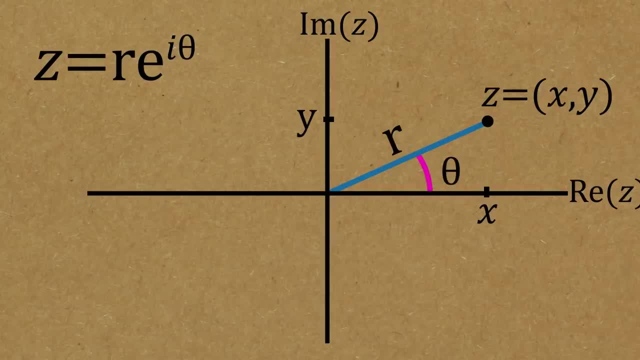 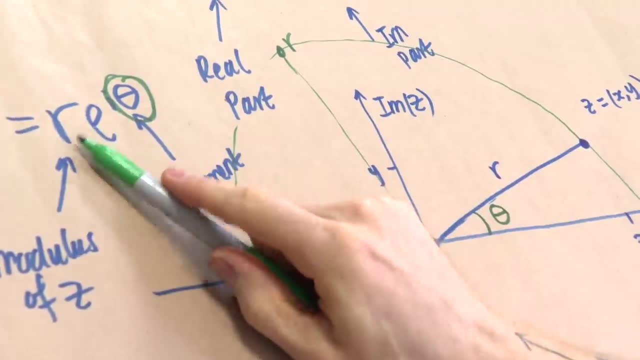 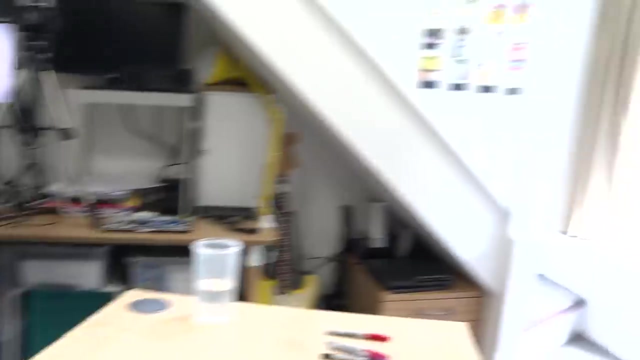 So we need to also give theta this angle, so we measure that from the positive x axis, like so. So if I specify the distance I am from the origin and the angle from the x axis, there's only going to be this one point, just like we uniquely had one point by specifying horizontal and vertical distance. 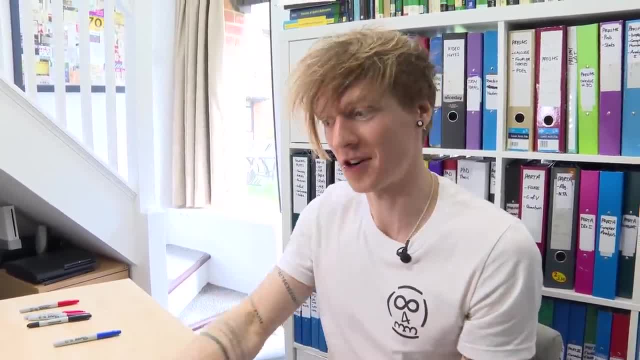 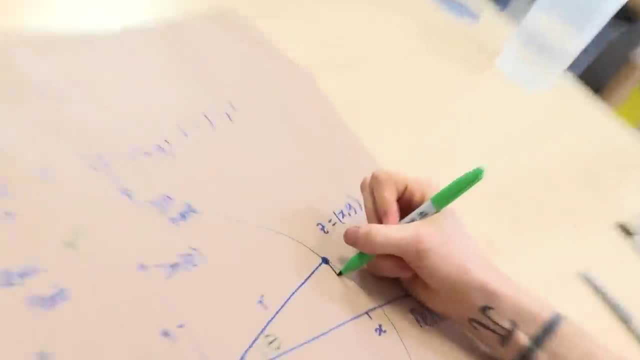 So now we've got two representations for our complex number z, So we want to compare them because they're the same complex number. And the way you do this is actually going to be by drawing a triangle, We drop that down, create a right angle. then we now know that this distance 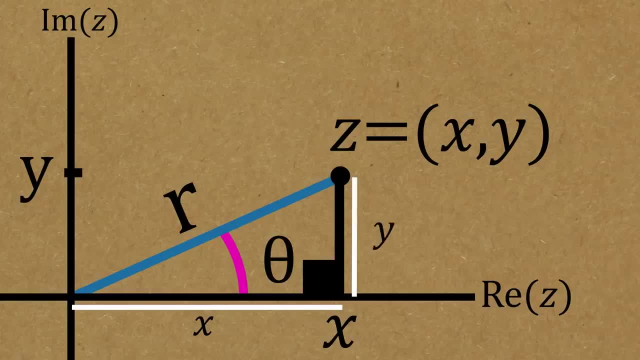 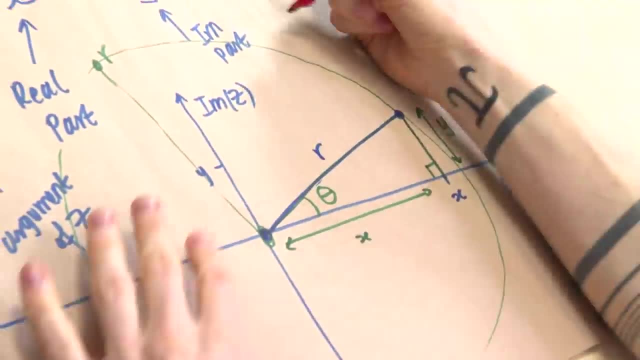 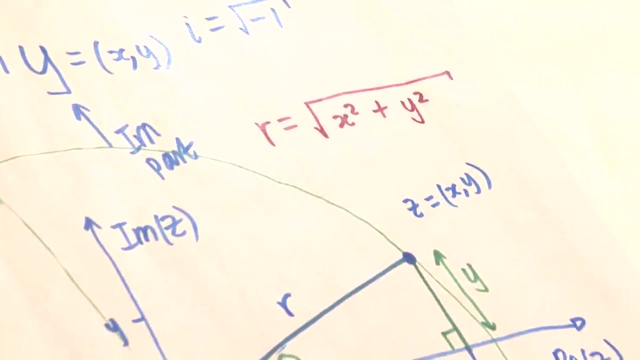 here is x, and we know that this height here is y, and then we know that our diagonal is r. So now we can use Pythagoras's theorem, which tells us that x squared plus y squared is r squared, So r has to be positive because it's a distance is equal to the square root of x squared. 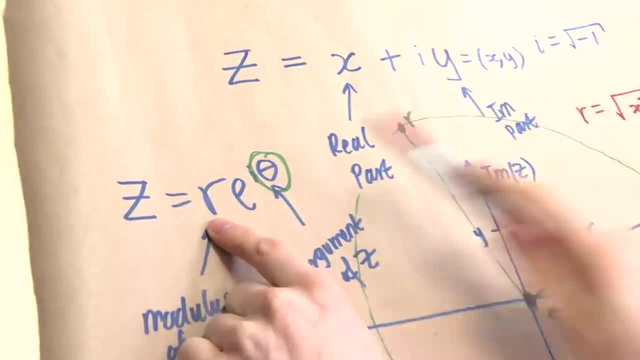 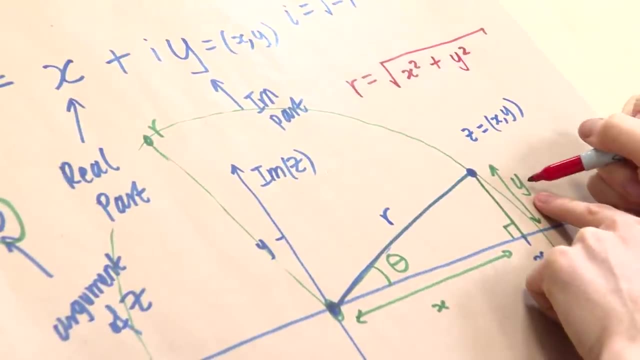 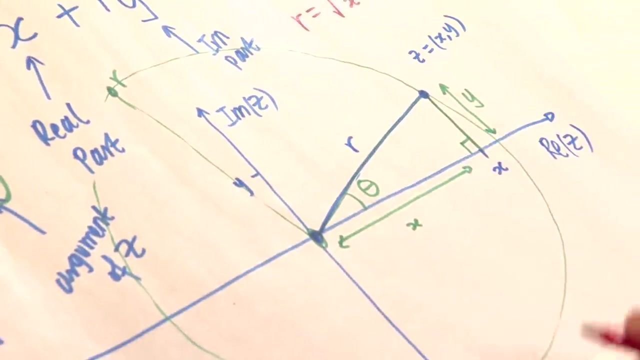 plus y squared. So we now, if we wanted, we could replace that by this, But what we really want to do is figure out what's happening with theta, Because, again, we know the height here and we know the horizontal distance and we know r, So trigonometry tells. 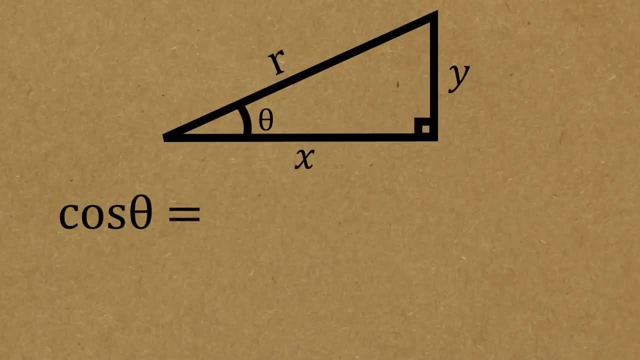 us that the horizontal distance is equal to the horizontal distance and we know r. So that tells me that cos of theta is equal to adjacent over hypotenuse, so that's x over r. Sine of theta is opposite over hypotenuse, that's y over r. So now we can actually say that x is equal. 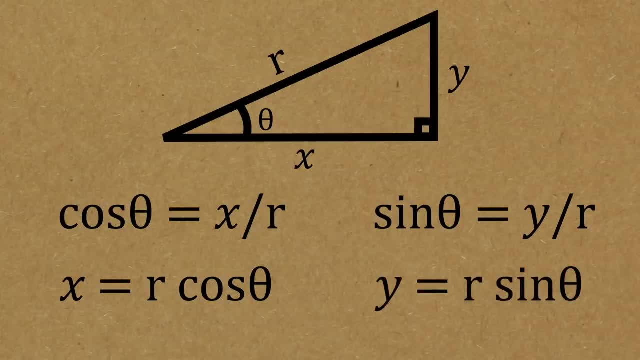 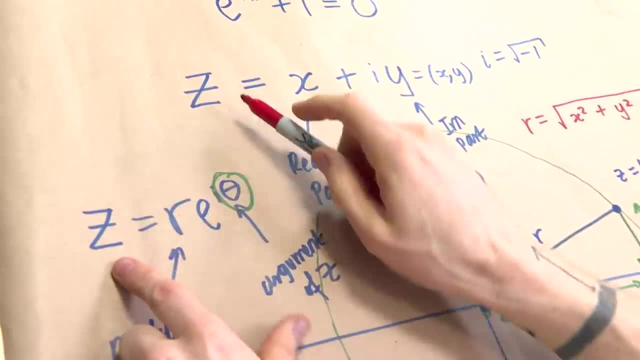 to r cos theta, and y is equal to r sine theta. So we've got these various relationships between x, y, r and theta and we have these two representations of z. But if we say this is the same complex number which on my picture it is, these all have to be. 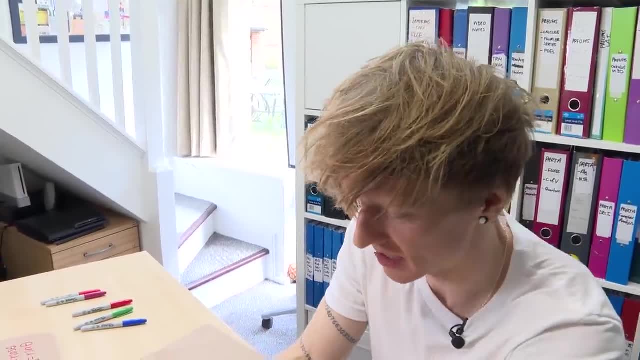 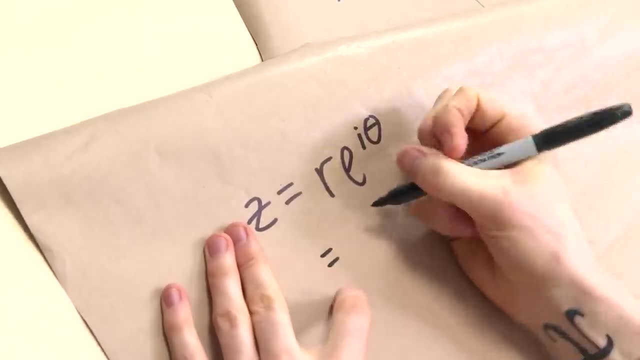 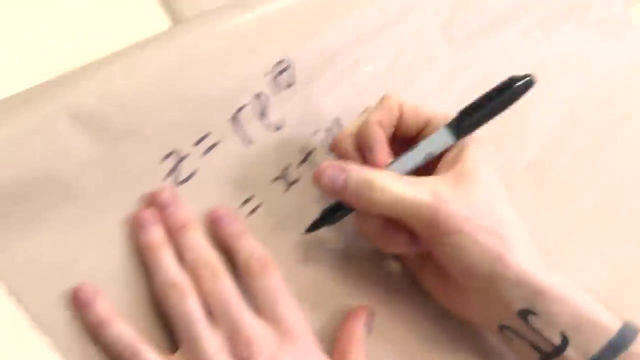 equal. So we have these two representations of z. so we know that z is equal to the distance times e, to the i theta, the polar form. We also know that this is x plus i- y. but we've got these two relationships for x and y, So let's plug those in and get r cos theta plus i times y. 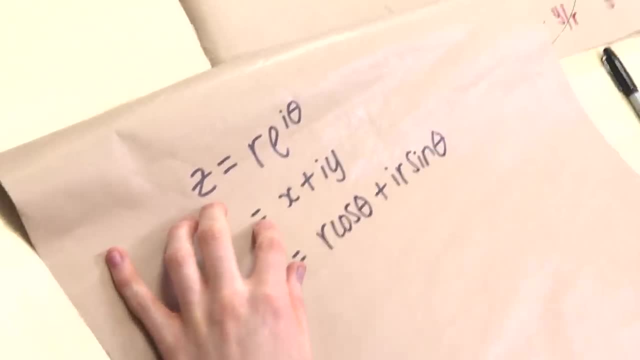 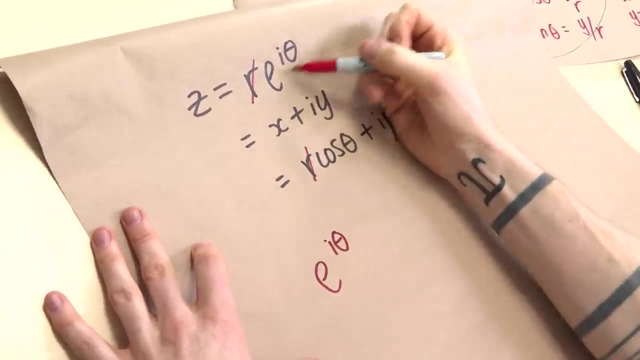 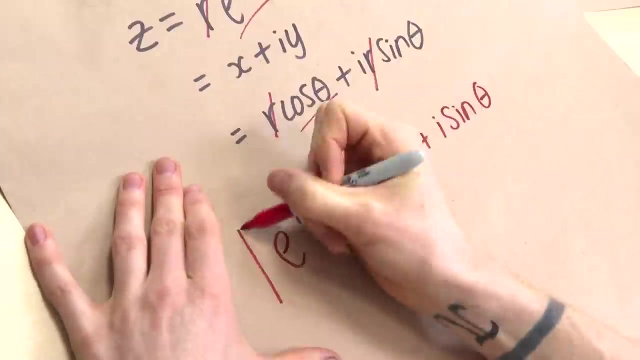 which is r sine theta. So if I now cancel the r, what I'm left with is this awesome equation, which is Euler's formula, which is that e to the i theta is equal to cos theta plus i sine theta. So that, right, there is Euler's formula, and it comes from complex numbers. 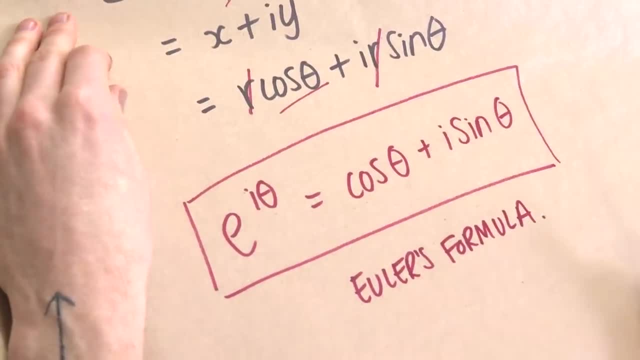 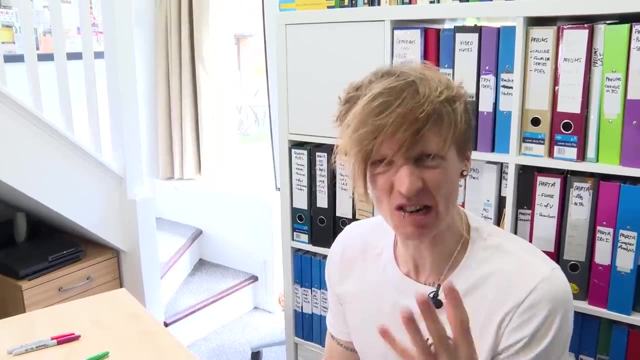 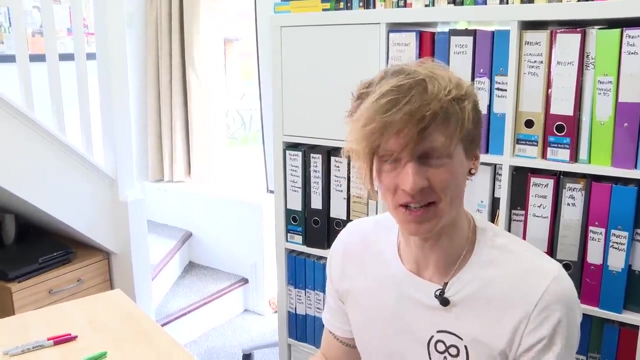 and just drawing out some triangles and figuring out some trigonometry. Now, Euler's formula is awesome. I love Euler's formula. There's loads of really cool stuff that we can do with this, and I'm going to show you three, I think, of my favorite things that we can do with Euler's formula. So we've seen where it. 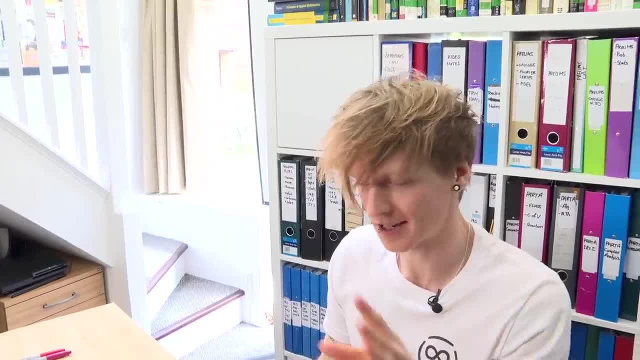 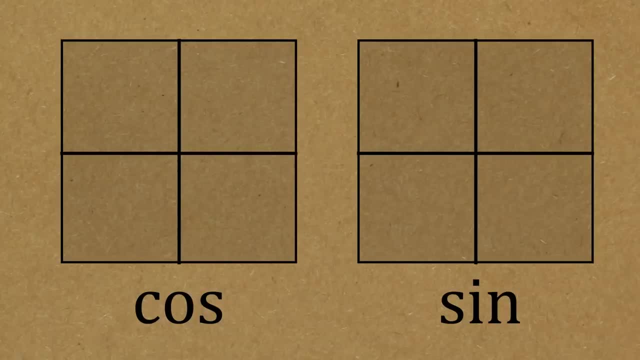 comes from. It's all to do with complex numbers, triangles, different things. Now we've got it. let's play around with it and see what we can figure out. The first thing that we're going to do is actually consider the graphs of sine and cos. So the cos curve starts at 1, comes down, goes up. 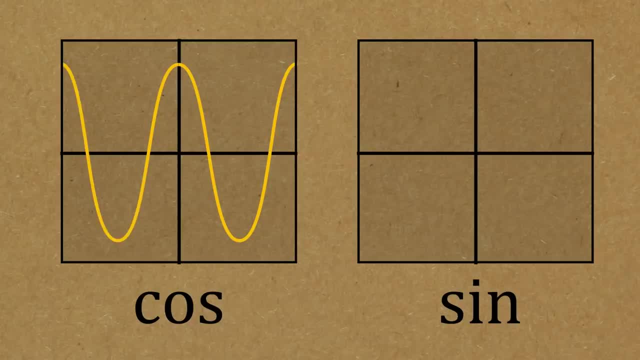 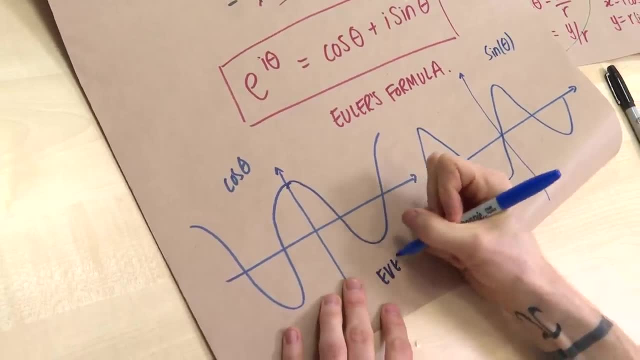 and similarly goes down and goes up, like that. And then sine, same shape but goes through 0, like that. Cos is what we call an even function. So this means that it's symmetric about the y-axis. So if you cover up that side, if you imagine putting a mirror here, you'd see the same thing. 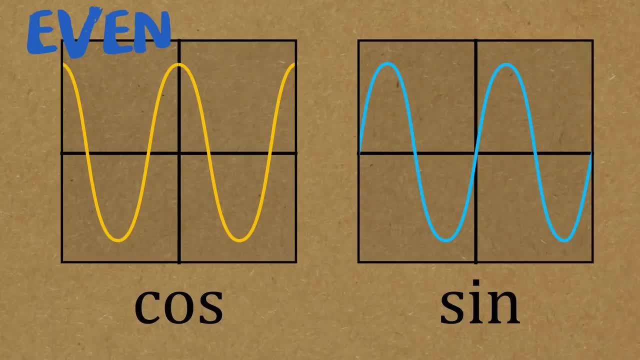 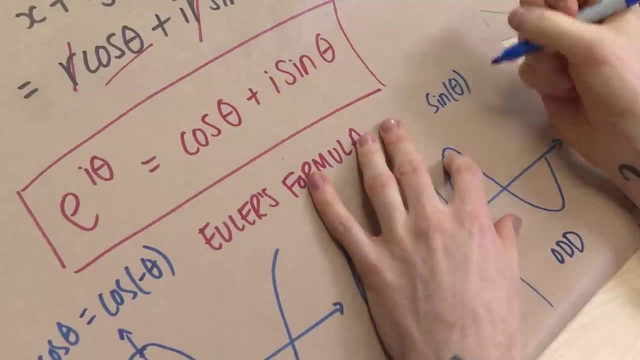 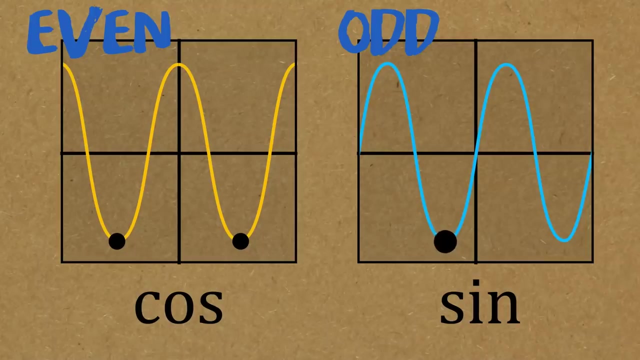 And this tells you that cos of positive theta here is actually equal to cos of minus theta. Now for sine. this is odd, and this tells us that sine of theta is equal to minus sine of minus theta. So if I look at this point down here, this is minus 1, so then minus minus 1 gives you a. 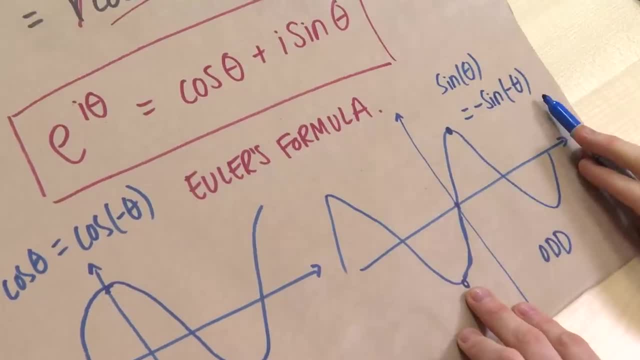 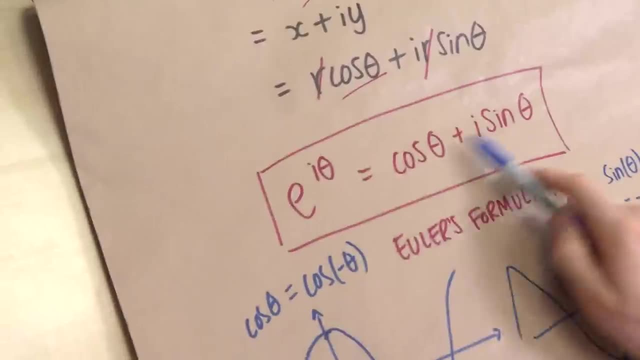 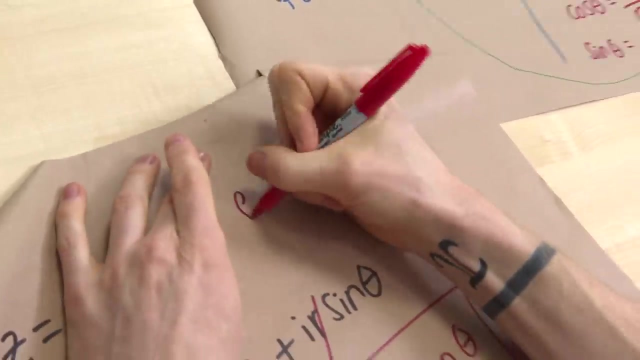 1, which is the one you get up here. So it's minus sine of minus theta. Now we can use these two relationships to get a really neat expression for cos and sine, because we've got this form for e to the i theta and if we look at e to the minus i theta. so what I'm doing really is I'm taking theta. 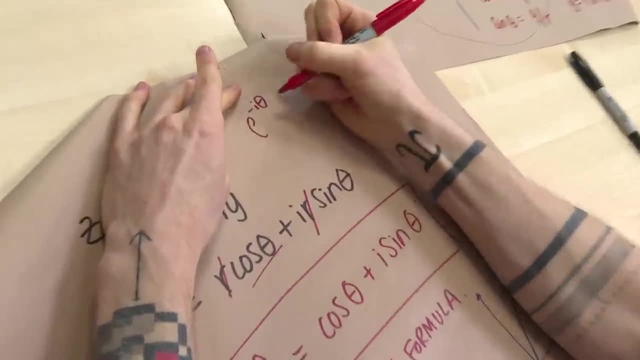 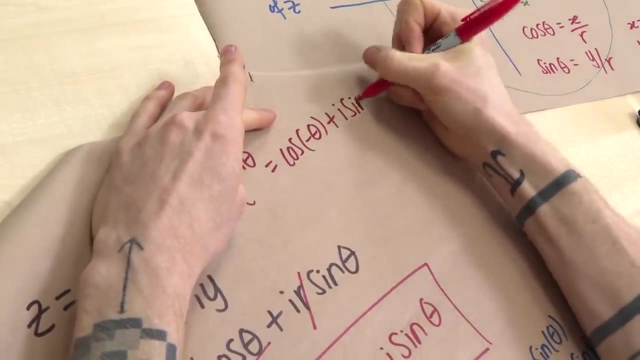 and replacing it by minus theta in the top, and then I do the same in here. So this is cos of minus theta, plus i sine of theta, Minus theta. So that's just taking Euler's formula: replace theta by minus theta in all. 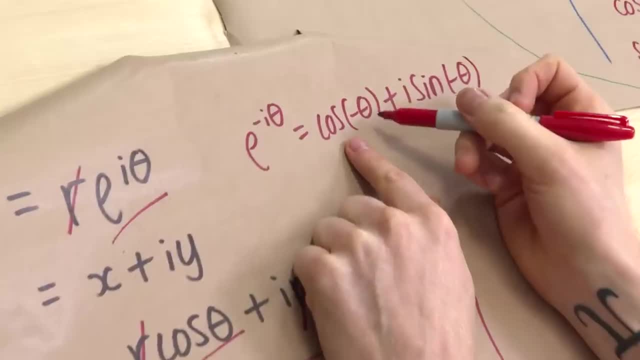 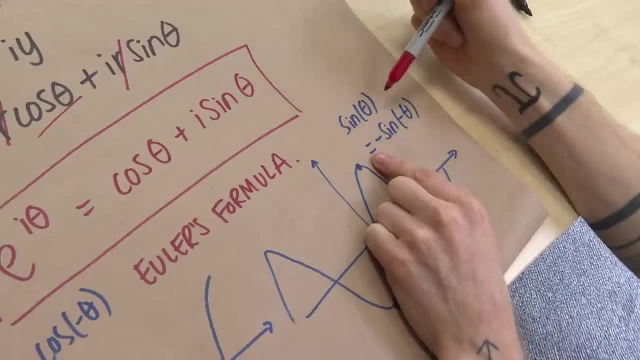 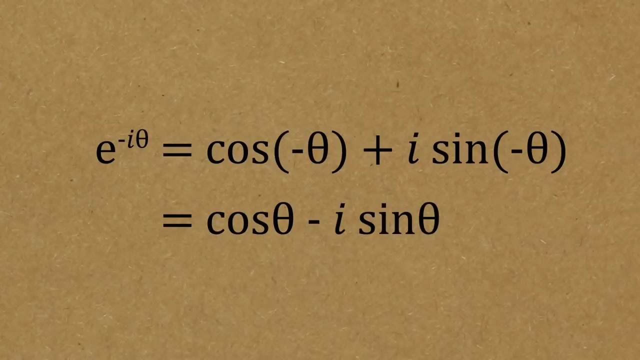 three places We have this result. But then we know that cos of minus theta, because cos is even, you get cos theta. Sine of minus theta, sine is odd. Sine of minus theta would be minus sine of theta, If I sort of do that, multiply by both, by minus 1.. So that's minus i sine of theta. 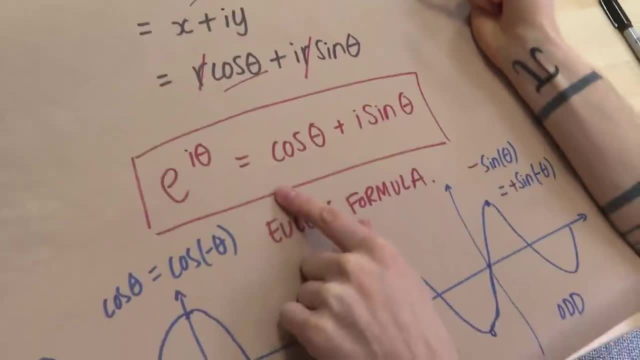 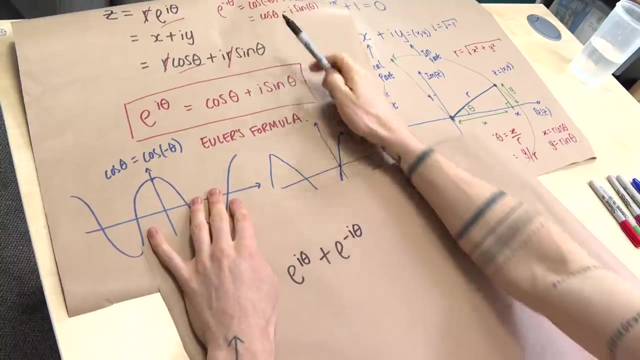 And now, comparing this equation and this one, we can add them together, So e to the i theta plus e to the minus i theta. So I've got a cos theta and then I've got another cos theta. So what I'm actually going to do is divide by 2, because I know what's happening. 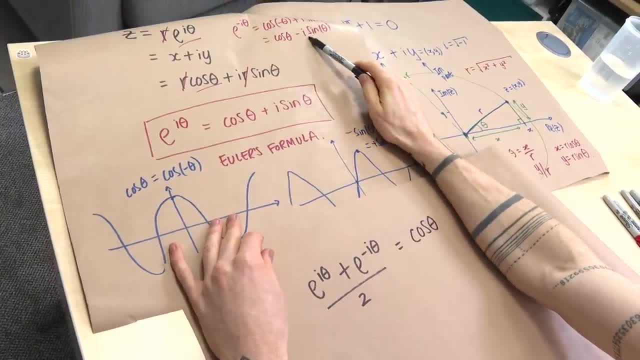 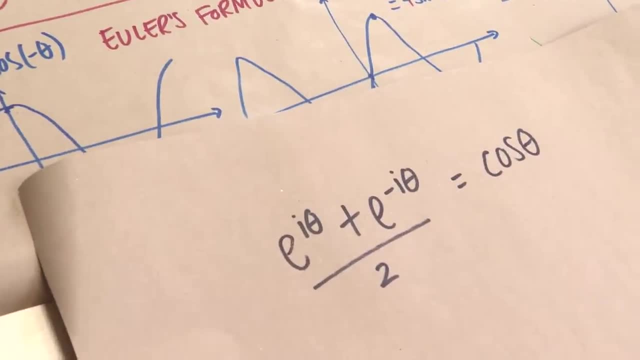 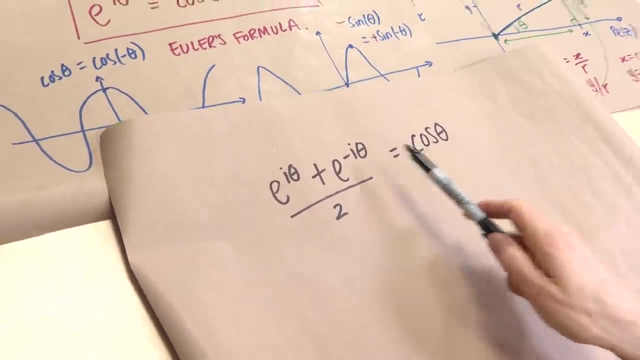 And that gives me single cos theta. And then I've got minus i sine theta, plus i sine theta, So they cancel, So I just get cos theta. So we've now got another definition for the cos function, this thing that we've seen the graph of and that we use in trigonometry. 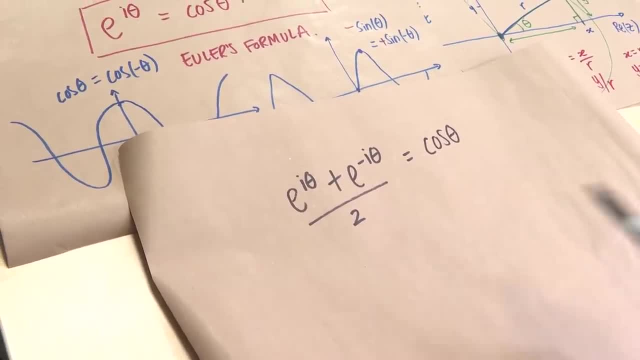 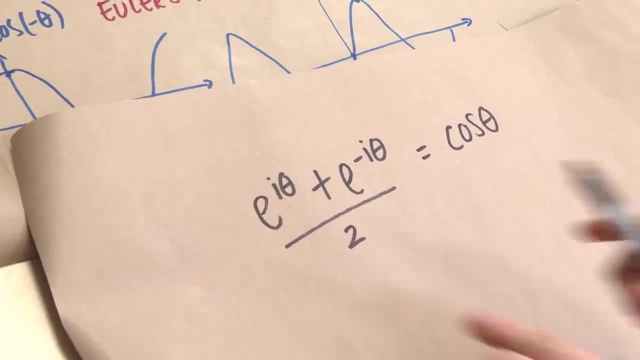 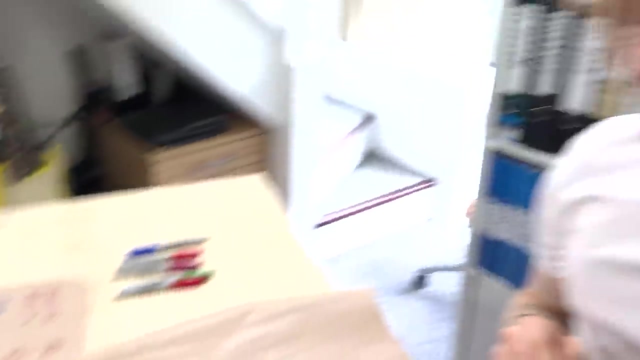 purely in terms of e and i, So it's a really nice. I really like this because you're taking this thing to do with triangles and this wave-like function and you're now expressing it in terms of Euler's number naturally appearing and also this imaginary number i. 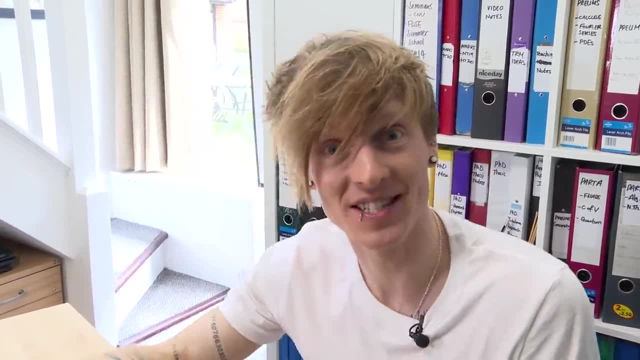 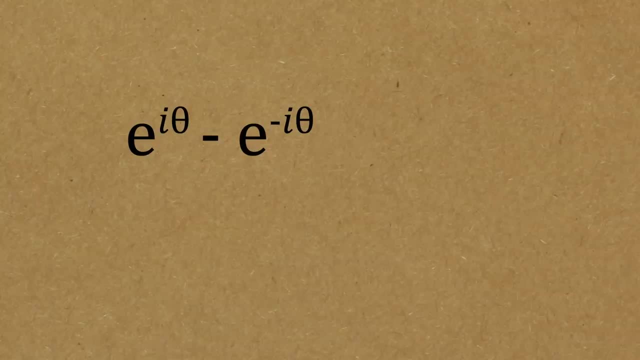 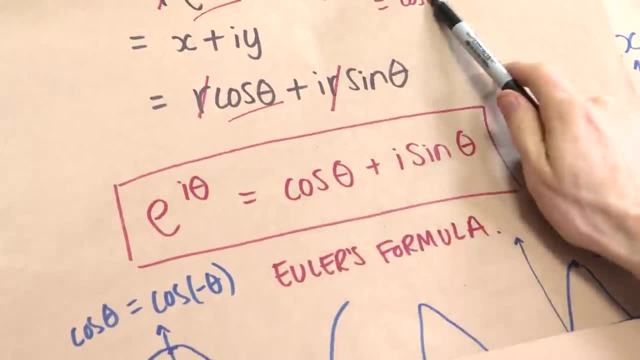 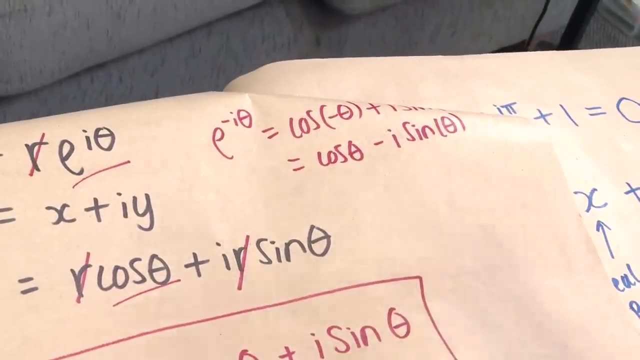 Minus i theta, because now that one's positive and that's now negative because we're subtracting this one, And then you've got i sine theta minus another one, so that becomes plus 2i sine theta. So you have to divide by 2i to get sine theta. 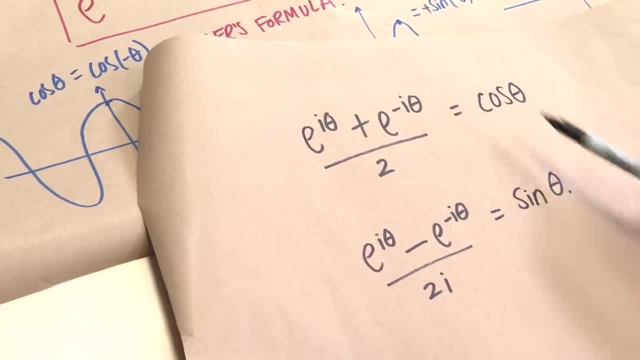 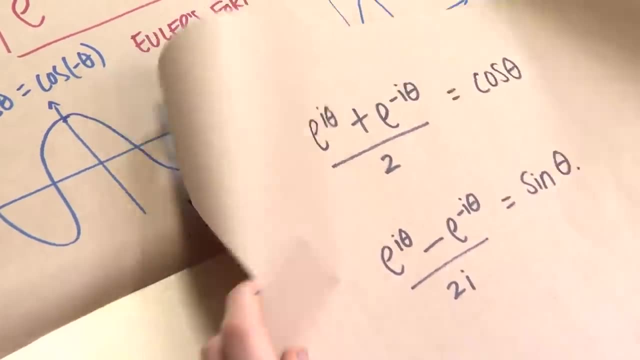 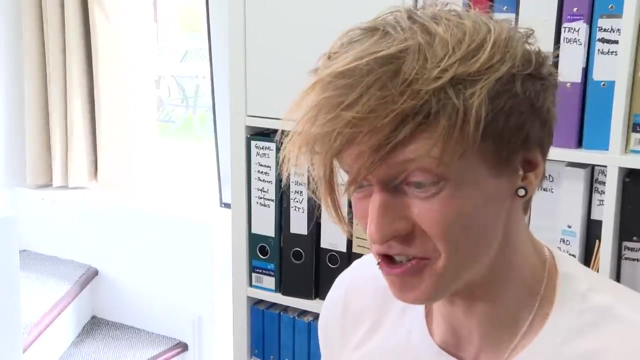 So we have a similar expression, So we can write cos and sine, both in terms of the exponential function. So that's my first favorite thing to do with Euler's formula. Now this leads us into my second favorite thing To do with Euler's formula, which is to do with infinite series. 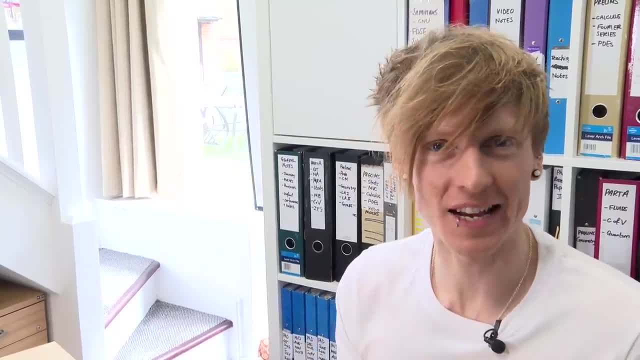 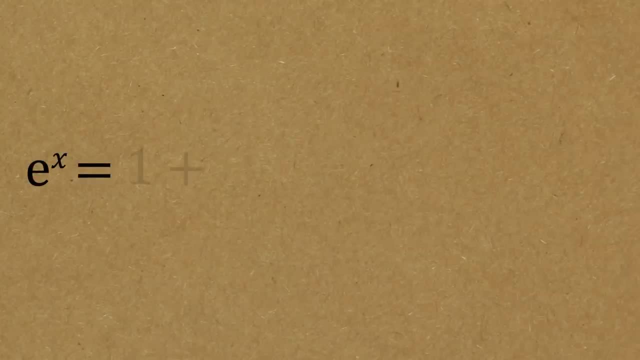 So we're going to start with the infinite series for the exponential function. I mentioned this before, actually in the video on domes e to the x, we can write as: 1 plus x plus x squared over 2 factorial, plus x cubed over 3 factorial, x 4 over 4 factorial, and this carries on forever. 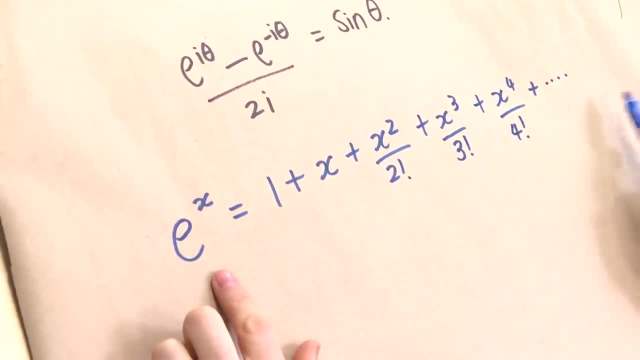 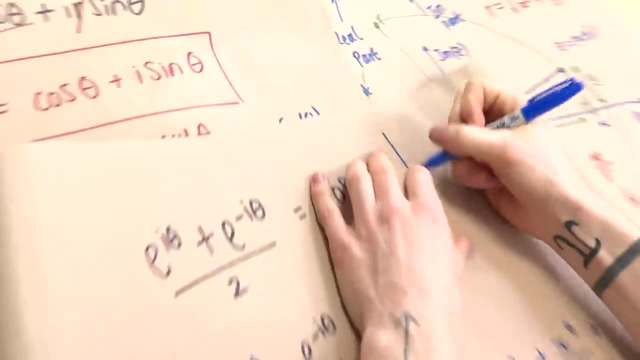 So this is just a way of writing out e to the power of some number. We can write it in this infinitely long string of pieces added together, And what this means is that the graph of e- because we keep adding things- starts really small, goes through one and then shoots up right Exponential growth. 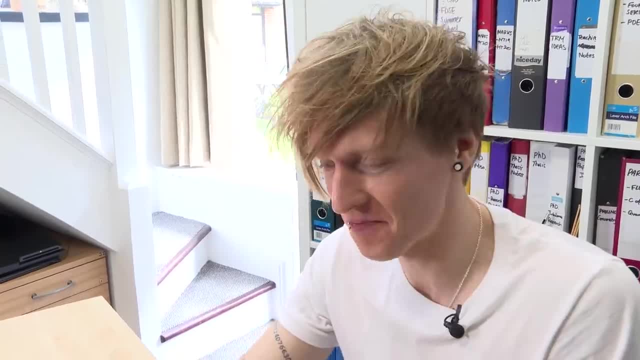 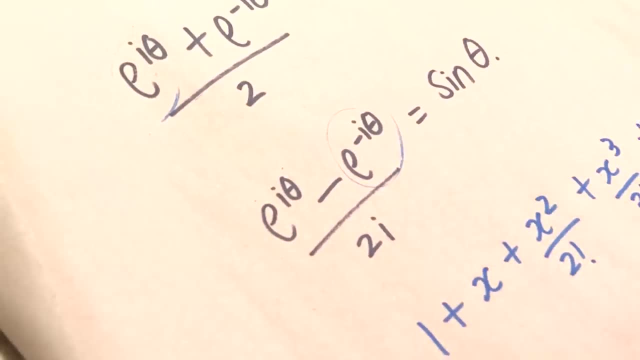 So that's what's happening with this function. Now we want to figure out what e to the i theta and e to the minus i theta are in this form, And then, if we add them together, the plan is we can now get infinite series for cos and sine- Another way of representing. 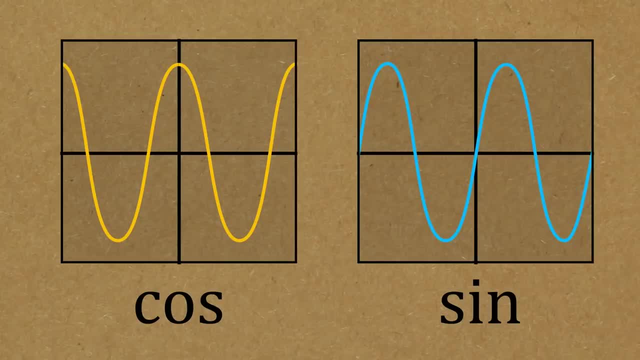 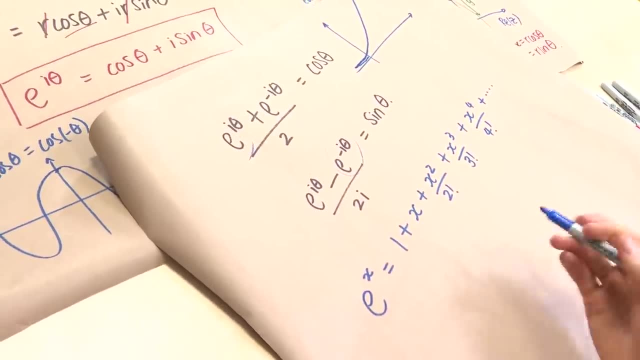 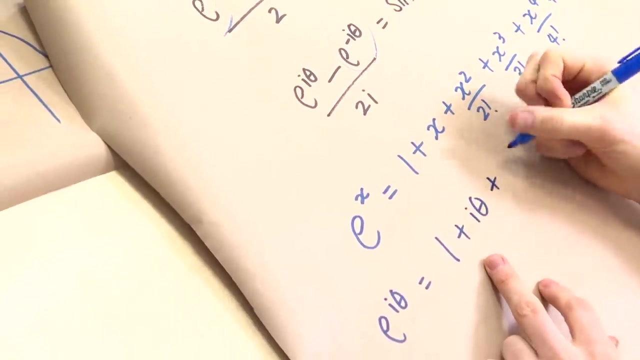 these cool trigonometric or wave-like functions as an infinite series based on what we have for the exponential here. So we need to calculate e to the i theta, So that's just going to be 1, then we replace x with i theta plus i theta plus i theta squared. 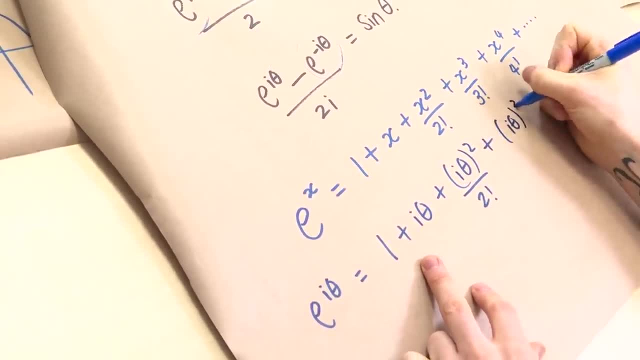 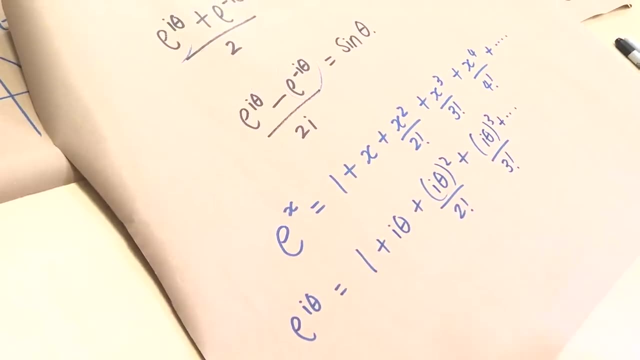 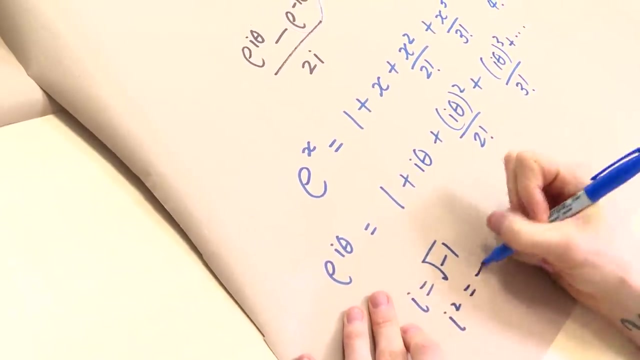 over 2 factorial, plus i, theta, cubed x, etc. And what we need to know is what's happening when we square and cube i. That's the key, Because we know that i is the square root of minus 1, so that means that i squared is minus 1.. 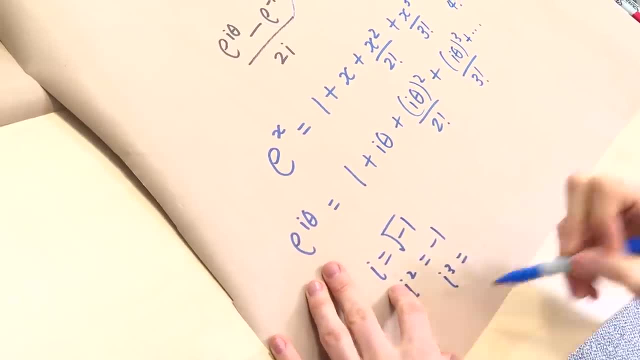 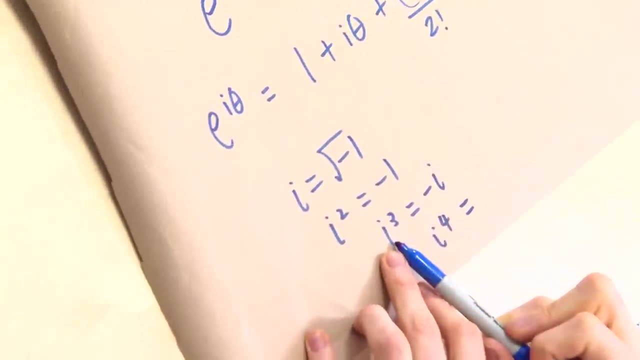 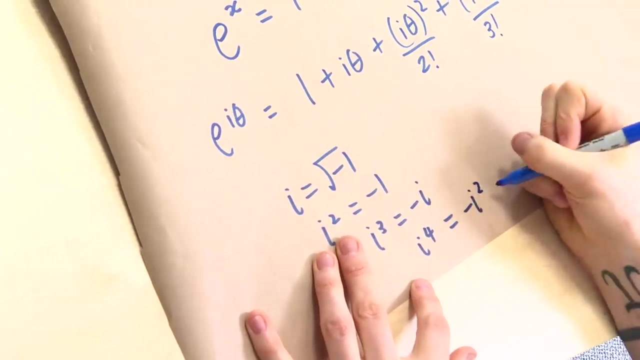 So that means that i cubed is i squared times i, so that's minus i. And then i to the fourth, that's i cubed times i, which is minus i, times i, which is minus i squared, which is 1, because i squared is minus 1.. 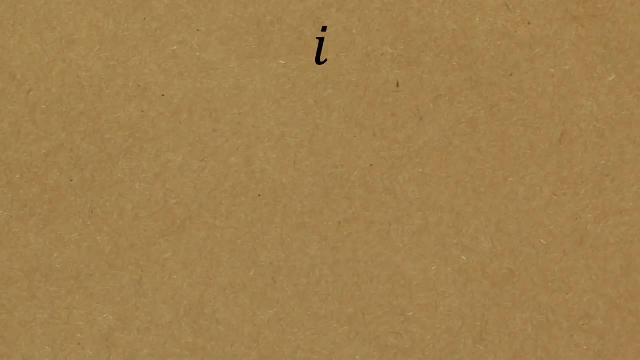 So we've got this little cycle between the numbers. So you start with i, then you multiply by i to go to minus 1, then you multiply by i to go to minus i, then you multiply by i to go to 1, because that was i- to the fourth. 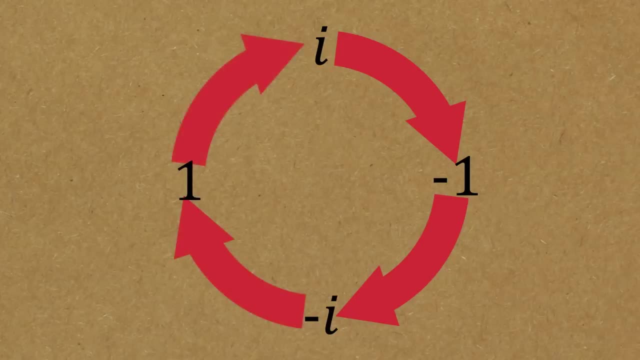 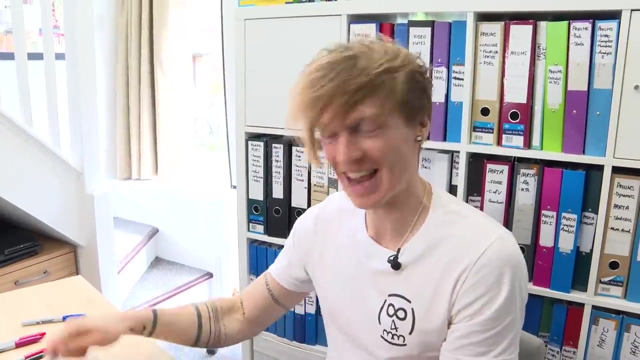 and then you multiply by i again, you get back there. So it actually creates a cycle. Every fourth power of i comes back on itself. So we can use this in our infinite expansion. So now we can plug this nice cycle into our formula. 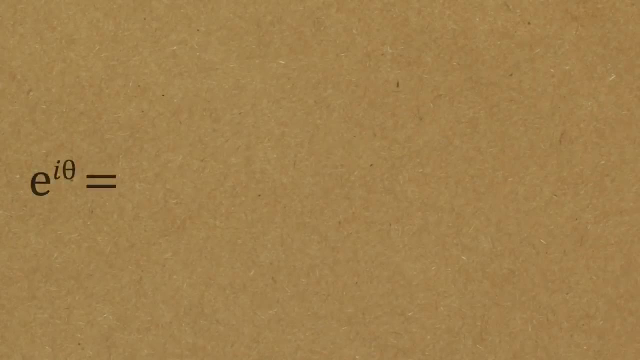 So what we're going to get is e to the i theta is: we've got a 1 plus i theta plus i squared. theta squared i squared is minus 1, so that's minus theta squared- 2 factorial. Then the cubed was minus i, so then it'll be minus i and we've still got the theta cubed over 3 factorial. 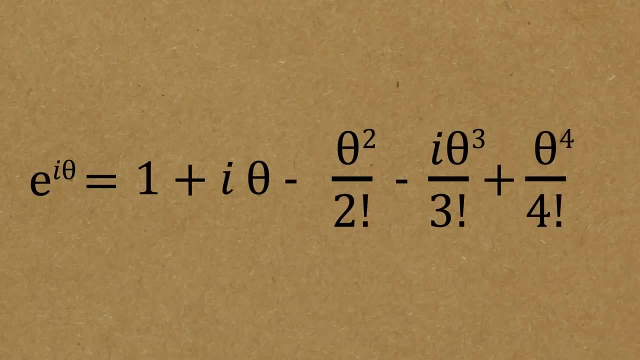 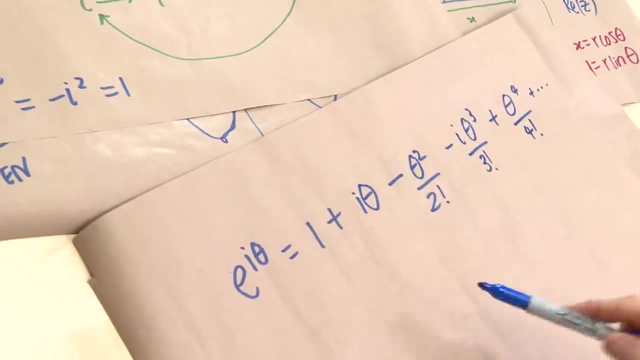 And then the last one. the fourth one was a 1,, so that's now plus theta to the fourth over 4 factorial, And then the pattern carries on, So the next one would have an i in front of it and be a theta to the 5 over 5 factorial, and then a minus, and then a minus, i, then a 1, and then repeating this cycle. 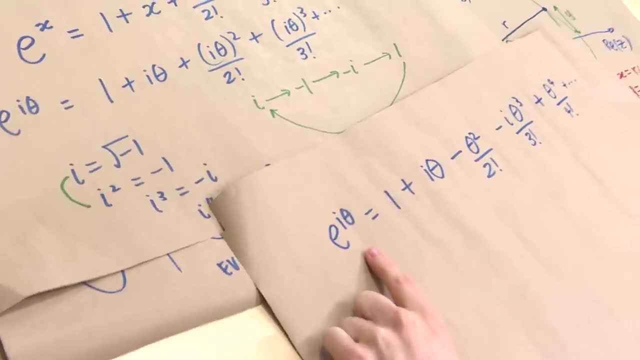 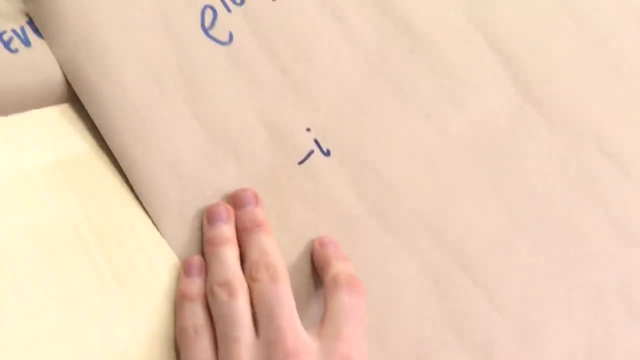 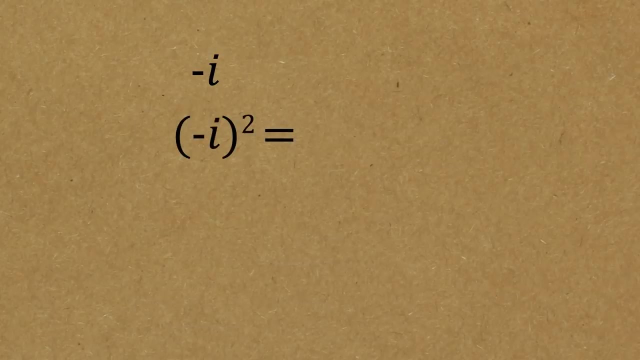 Now we want to do the same for e to the minus i theta, And in order to do that we need to know powers of minus i. So we've got minus i. then we want to now do minus i squared, So that's minus i times minus i, which is going to be plus i squared, which is minus 1.. 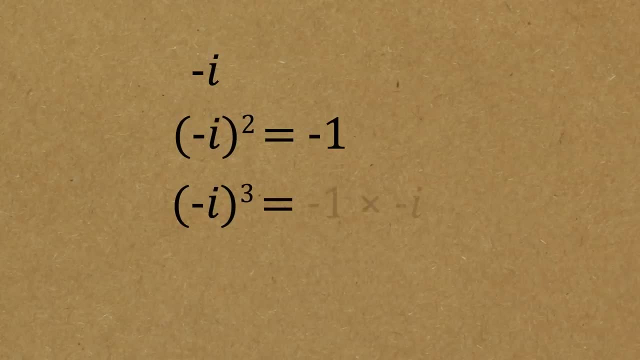 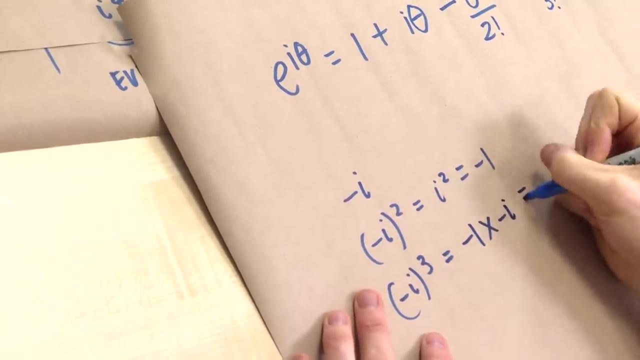 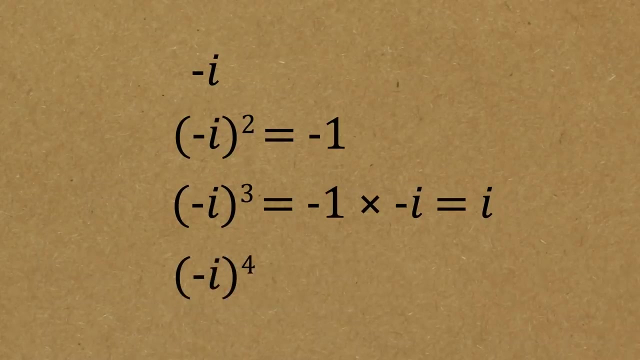 Then we've got minus. i cubed is minus 1.. So that's minus 1 times another minus i. so that gives me a minus 1 times a minus 1, I'm going to write this out: minus 1 times minus i. so they give you a plus, so that's just i. and then we multiply again. minus i to the fourth is going to now be minus. i squared which is minus minus 1, which is 1, and then we're going to get back again. 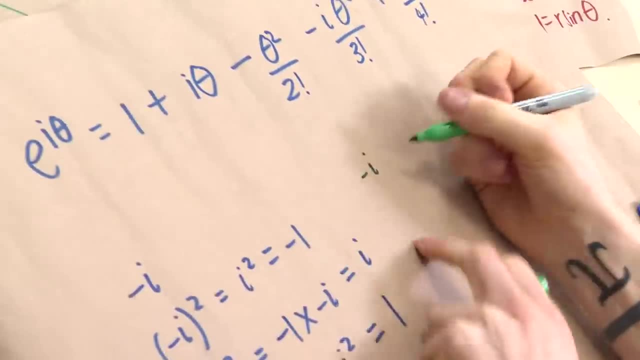 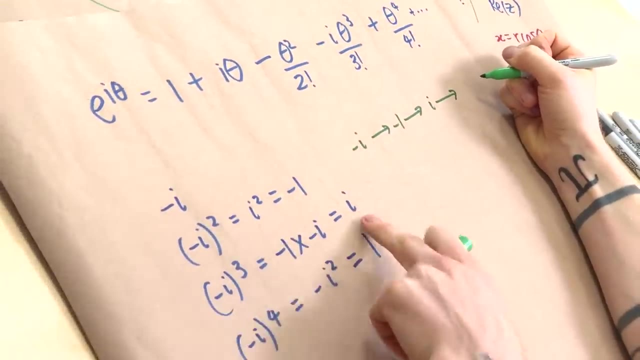 So, just like before we start at minus i, we multiply by i to get minus 1, we multiply by i to get i, and again, by sorry, by minus i to get i, And then by minus i to get 1, and then by minus i to get back. 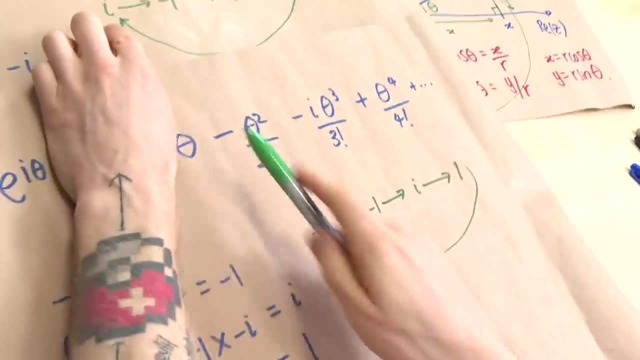 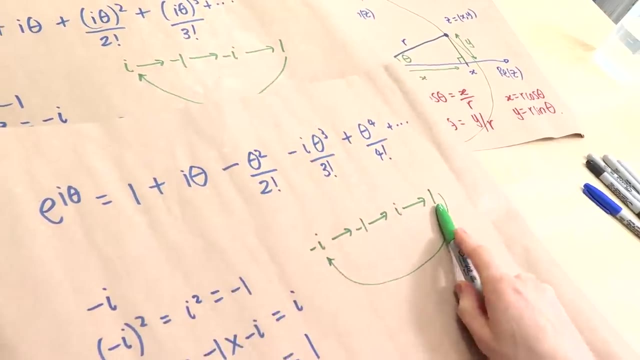 So it's the same kind of idea, except two key things. This started at i, this starts at minus i. then it's the same. Those are different, that's the same. So in our formula what we're going to get is e to the minus i theta is 1 minus i theta. 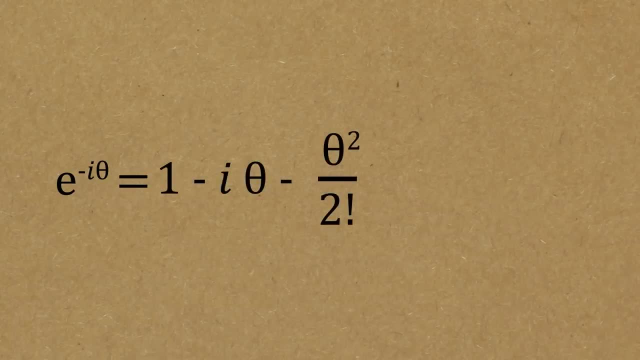 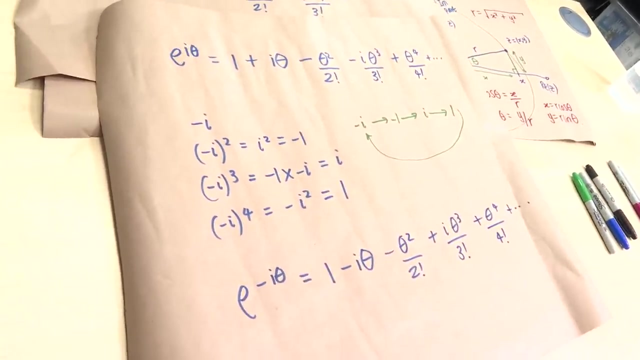 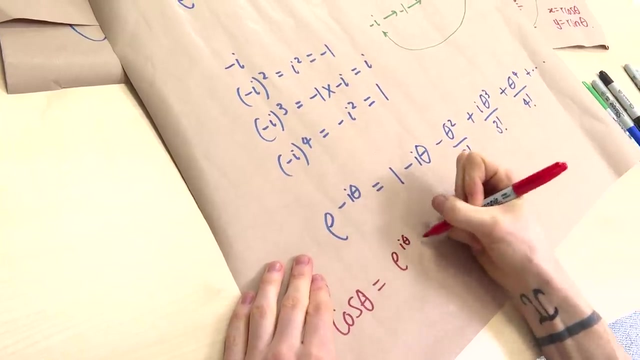 Then it didn't change, so it's still minus theta squared over 2 factorial. Then it was now plus i theta cubed over 3 factorial, And then plus e to the fourth over 4 factorial, and the pattern repeats. So now the big result, what we were trying to get with our infinite series is we said that cos theta was e to the i theta plus e to the minus i theta over 2.. 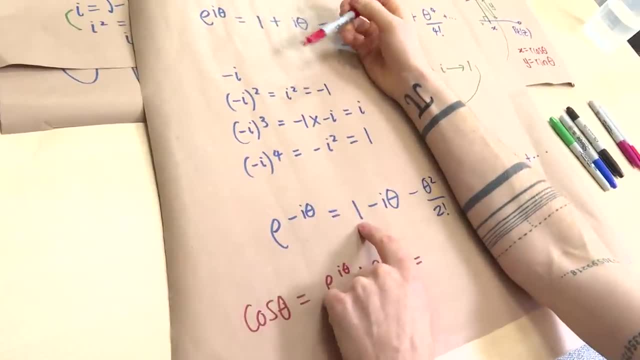 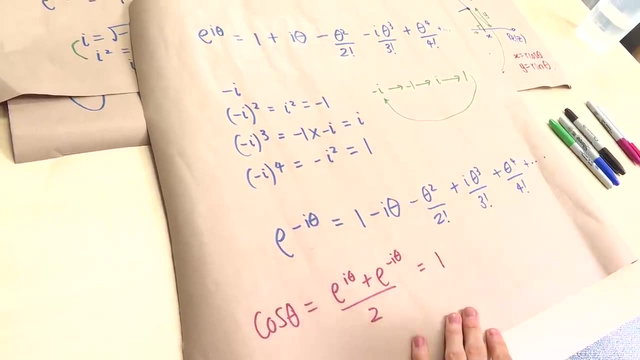 So let's add them together. So 1 plus 1 is 2, divided by 2,: 1.. i theta minus i theta is 1.. i theta minus i theta is 1.. i theta minus i theta disappears. 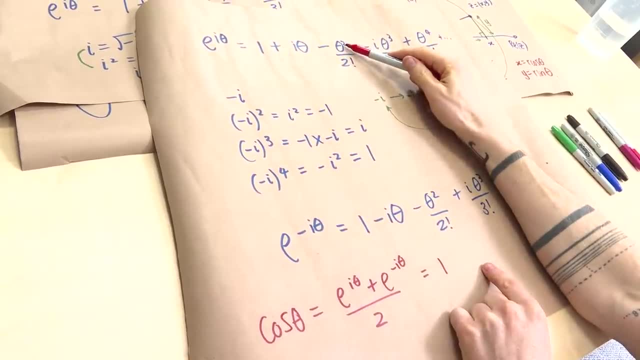 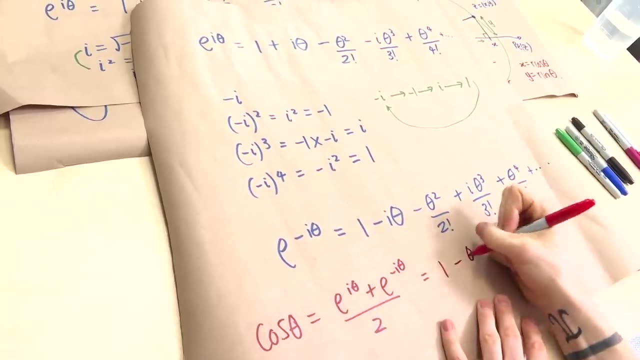 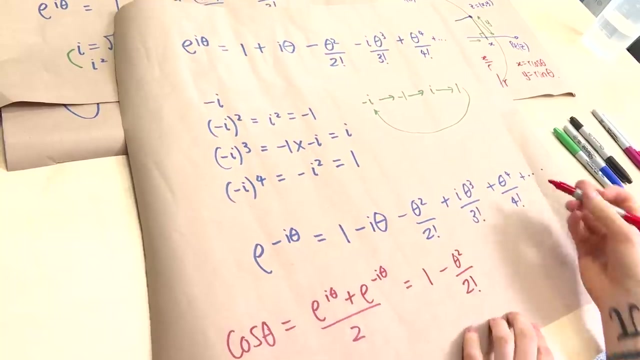 So we get no term there. Minus theta squared, minus another theta squared is minus 2 theta squared, but then we divide by 2, so I get minus theta squared, 2 factorial Theta cubed term: cancel opposite sign. and then we get theta to the fourth over 4 factorial. 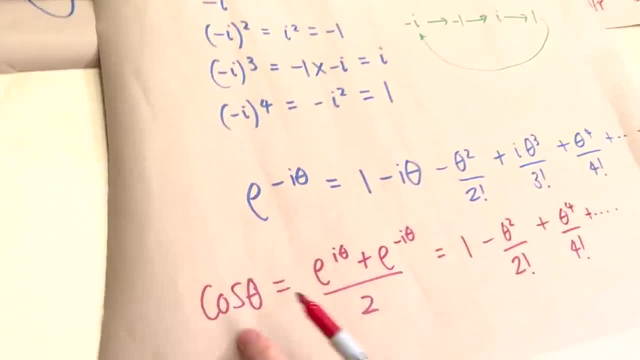 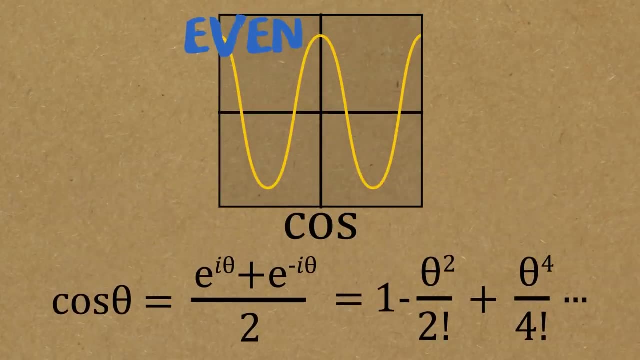 And this carries on. So what we're seeing here is the cos term has all of the even powers of theta, And there was a bit of a clue earlier when we had the graph of cos, when we said it was even. This doesn't prove it by any stretch, but even and even it's nice. 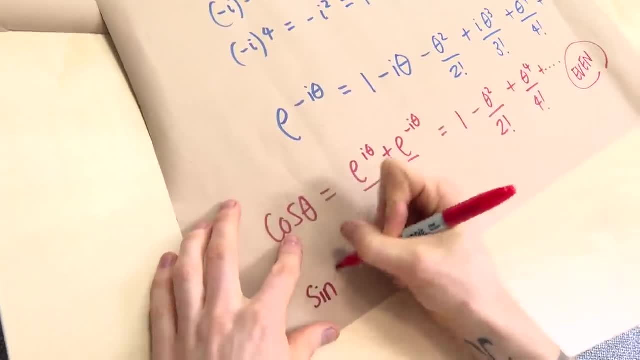 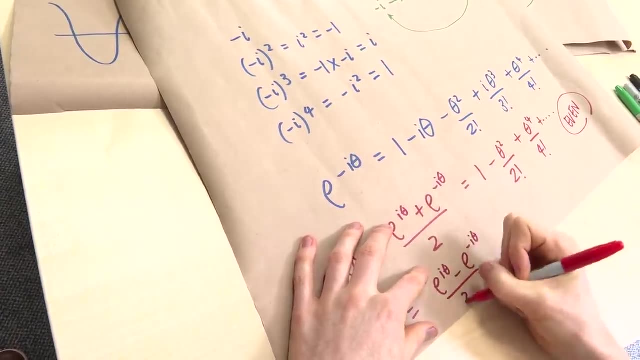 So we've got all the even powers for cos and we do the exact same with sine of theta, But this time we do e to the i theta minus minus i theta over 2i. So the first term they subtract each other to give 0. 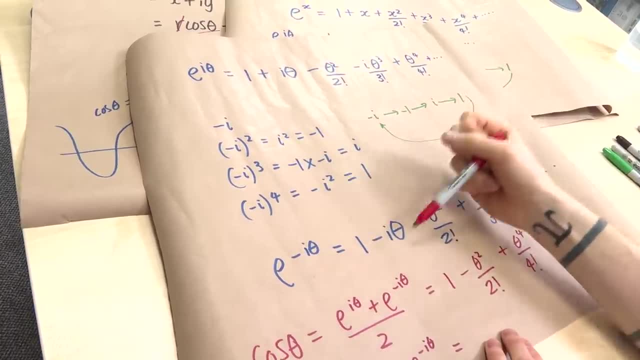 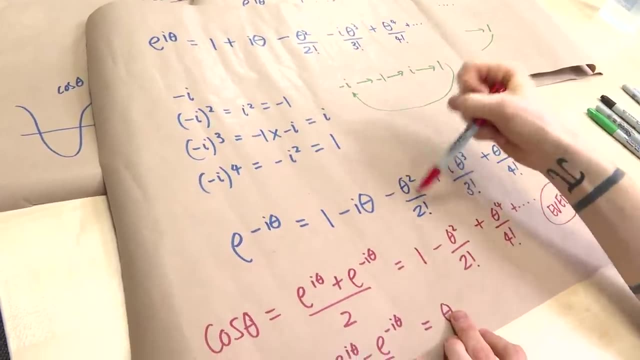 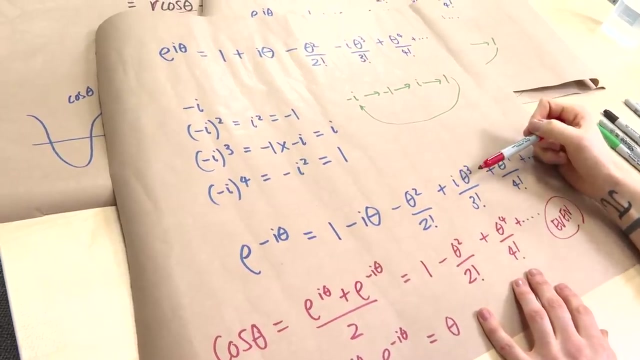 This one minus this one gives me 2i theta Divide by 2i. so I just get theta. That one minus this one comes a plus. so they cancel: Minus i, minus another i, so that gives me minus 2i theta cubed divided by 2i. 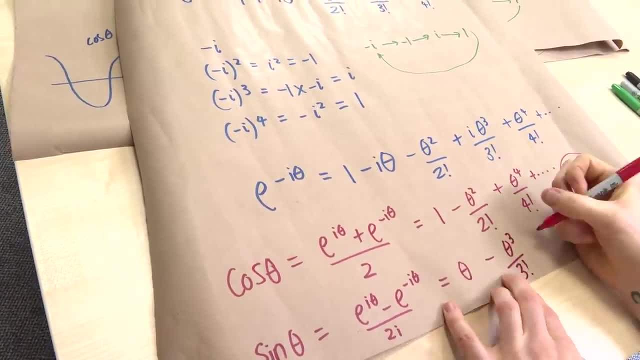 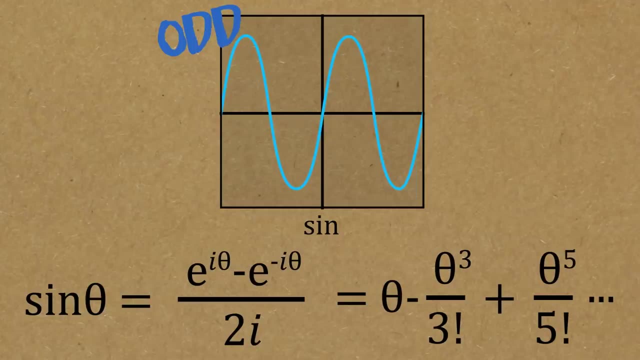 So I get minus theta, cubed over 3 factorial, And then that will carry on as well in the same way. So we get power 1,, power 3,, power 5. We get all the odd powers for our sine series. 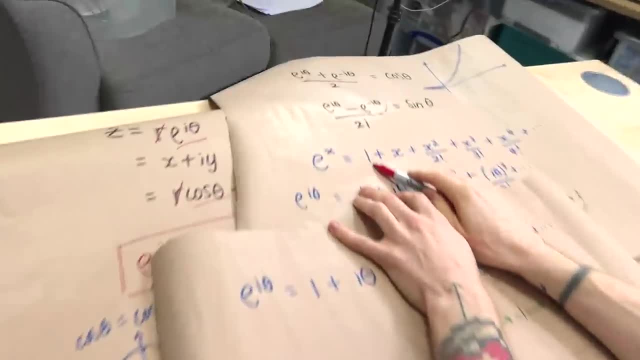 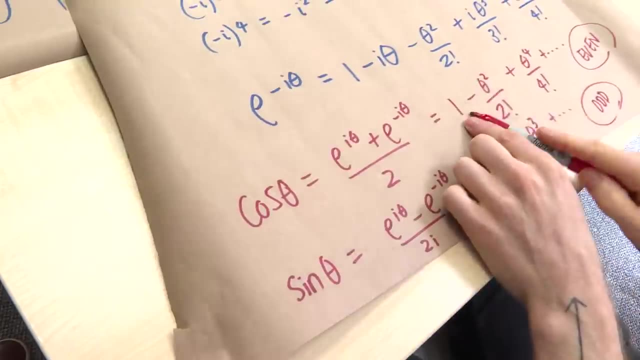 So, just like the exponential term is written here, It has 1 plus x plus x squared cubed, divided by the factorials Cos, and sine cos is all of the even powers. where you alternate It goes minus, plus, minus, plus, minus plus. 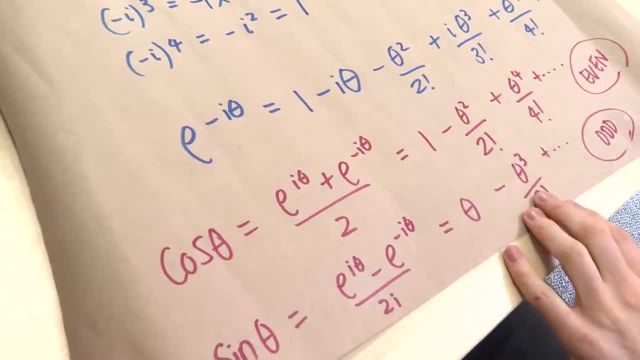 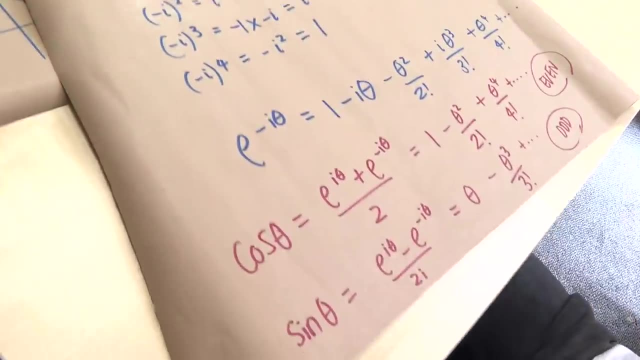 And sine is all the odd powers going plus, minus, plus minus, plus minus. So from the infinite series for the exponential function we now get these nice infinite series for cos and theta, And this is why sine of theta is often approximated by just theta if you're an engineer. 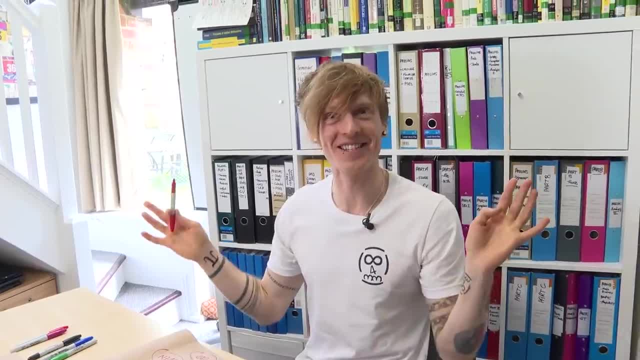 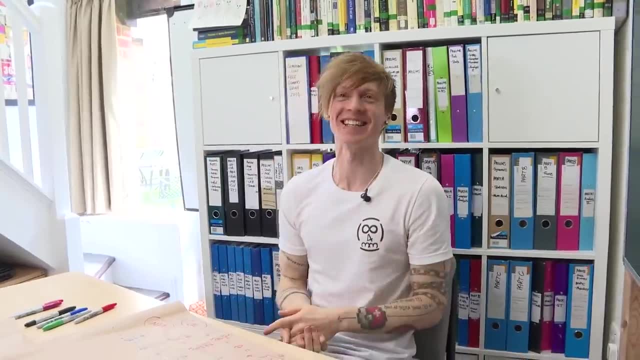 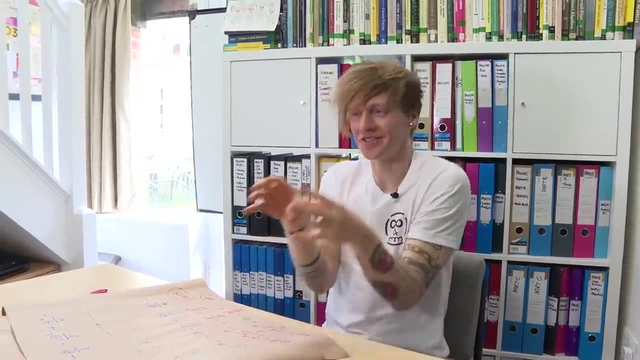 Because it's the first term in your infinite expansion. All right, You seem excited by that. I love infinite series. I think infinite The fact that you can take this function that looks like a wave or this function that's to do with triangles. 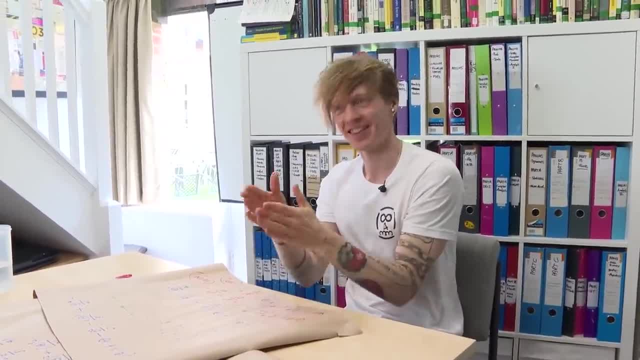 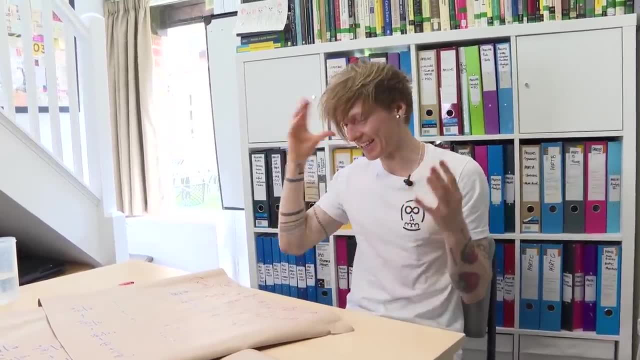 and write it as an infinite things added together. it still blows my mind Like I know it's true because I've just hopefully convinced you that it's true, But it's still I don't know. It's just things like this with maths that excite me. 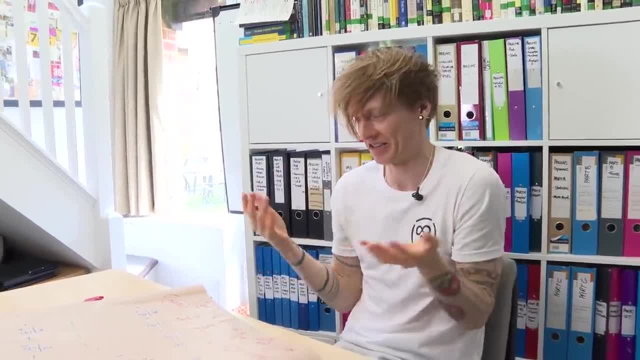 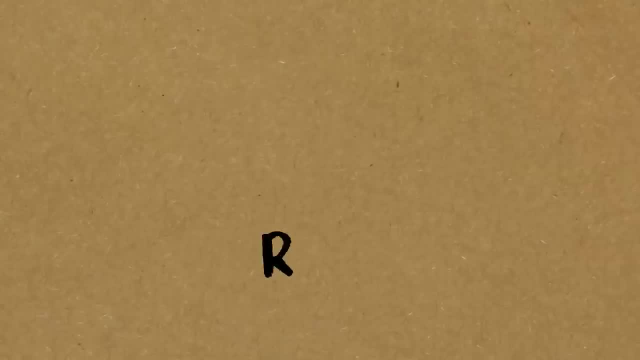 Like talking about infinity and it actually making sense. I think it's just really amazing. we've been able to do this. So the big finale: actually Should we get one final piece of paper, More paper. So we've seen, hopefully, some really cool stuff involving Euler's formula. 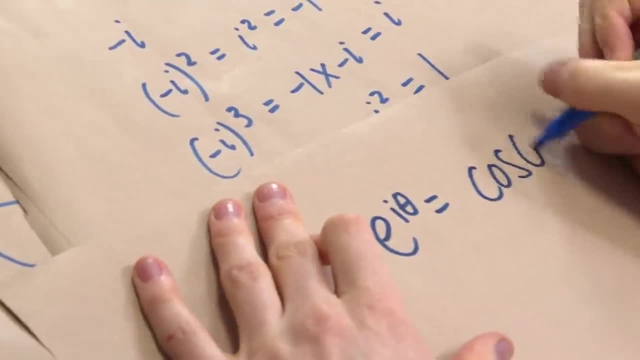 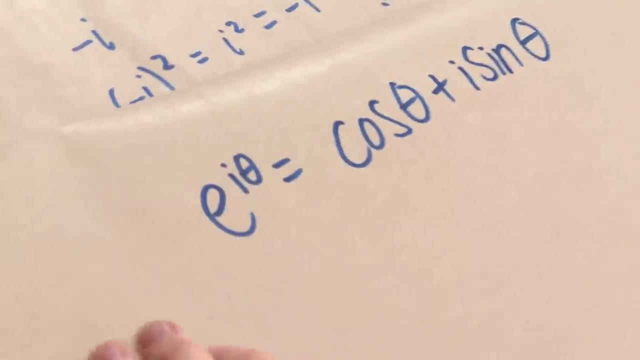 We derived it e to the i theta using complex numbers. We showed this was cos theta plus i sine theta. We then played around with some infinite series and I got very excited. And now what we want to do? I did promise you we were going to do some cool stuff around Euler's identity. 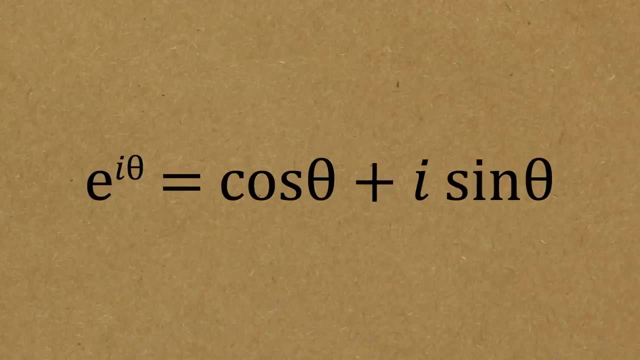 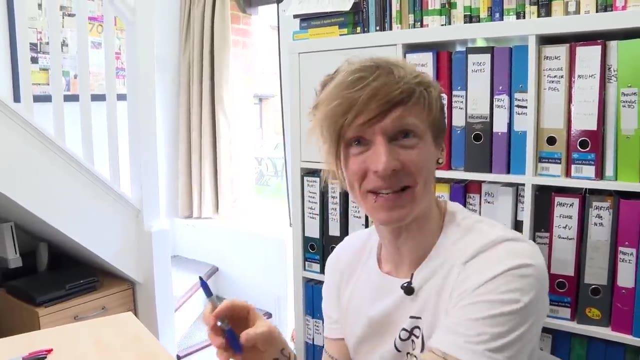 So this is the key. Euler's formula is really the foundations behind Euler's identity. Euler's identity is like the pretty facade of the building that everyone loves, But the heavy lifting is being done by Euler's formula, And to get it you just substitute in a value of theta. 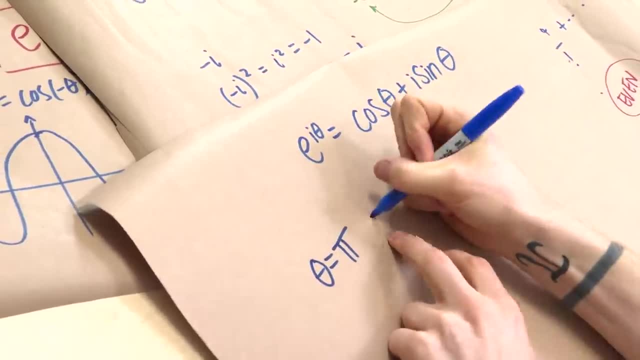 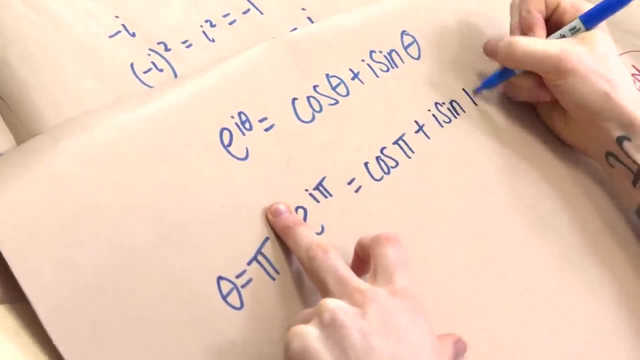 You just plug in: theta equals pi. So e to the i pi is equal to cos of pi plus i times sine of pi. And now if we look at our graphs, we can read off the value of cos. Cos of pi is minus one. 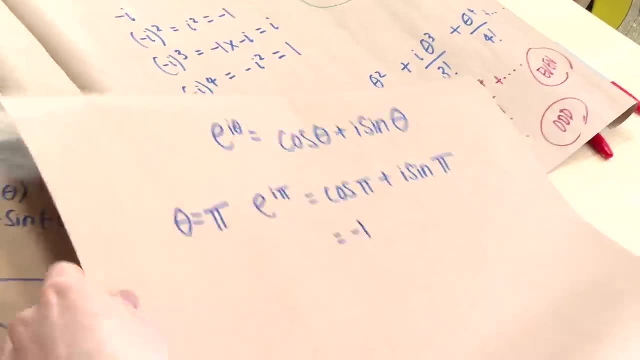 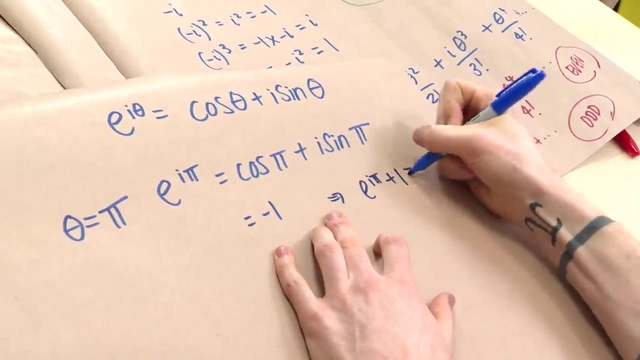 Sine of pi is zero. So e to the i pi according to Euler's formula is minus one, which we rearrange to get. e to the i pi plus one equals zero. Euler's identity. Now, that's my favorite form of it. 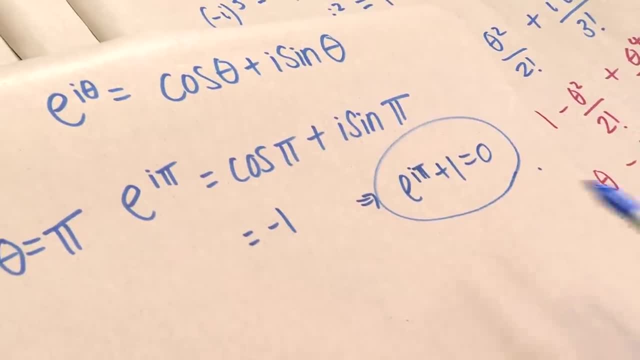 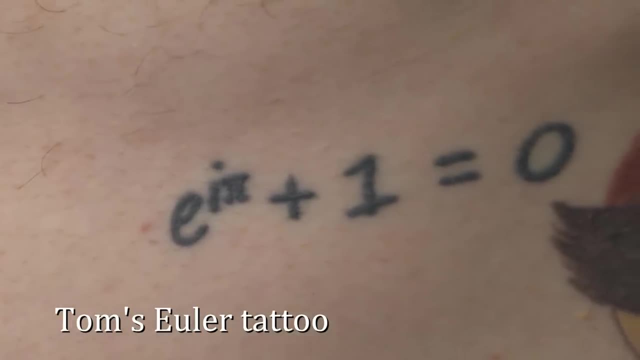 Some of you might prefer the e to the i. pi equals minus one, but I quite like getting the zero in there. Yeah, it needs a zero for me, I agree. I agree, This is the one I got tattooed. This is the one. 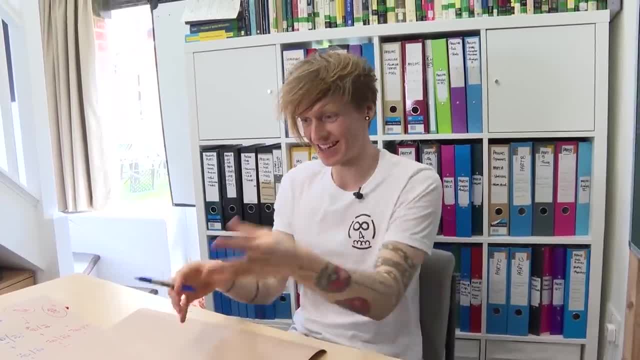 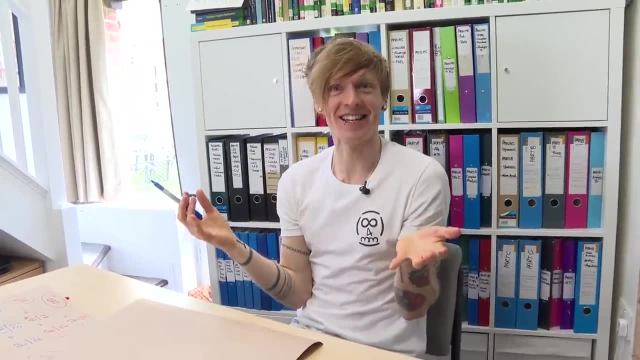 Now you can plug in other values of theta. This is why I wanted to share with you all Euler's formula, because you can plug in any value of theta and create your own identity of this kind of form. We can plug in pi by two, which is 90 degrees. 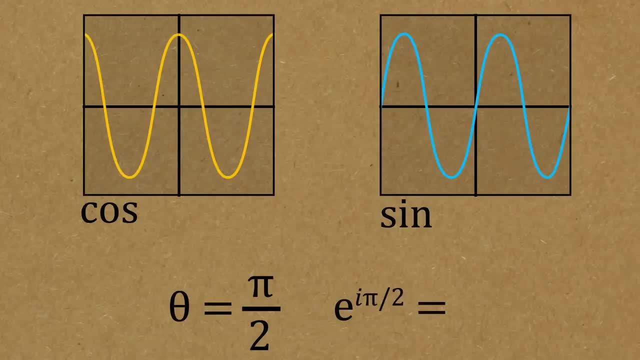 And we get e to the i pi by two is cos of pi by two. Well, that's zero. And then plus i sine of pi by two. sine of pi by two is one, So e to the i pi by two, So e to the i pi by two is i. 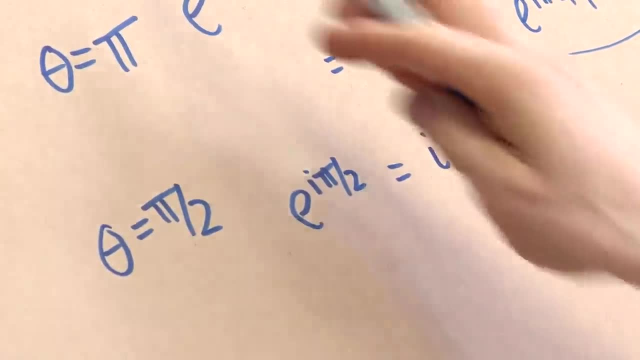 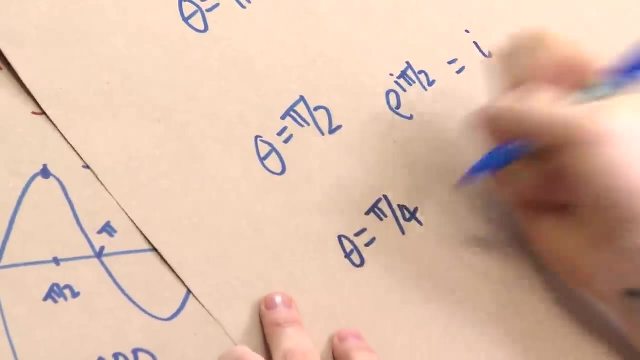 So that's a nice alternative definition of i, which has come from the same formula as Euler's identity did. We can then try 45 degrees, So that's pi by four. So that's halfway up here. So e to the i, pi by four equals cos of pi by four. 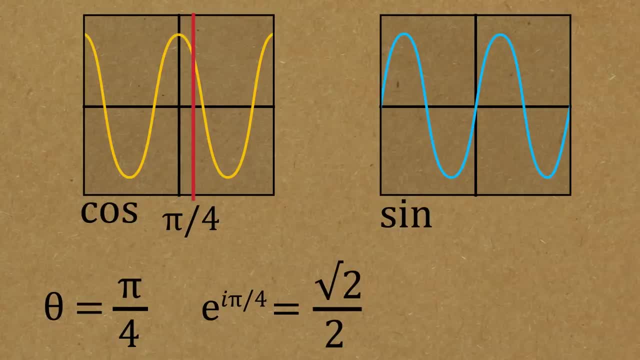 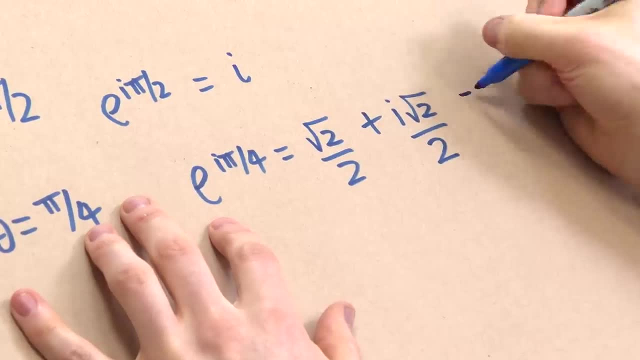 which is root two over two, And then sine of pi by four, is actually the same value, And this is very nice, because this number is actually equal to the square root of i. i to the half, Because what you do is you take this formula. 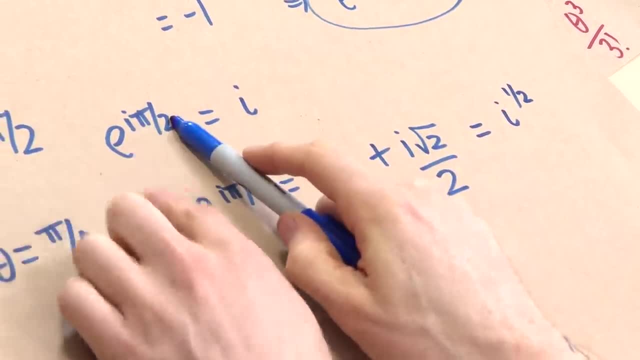 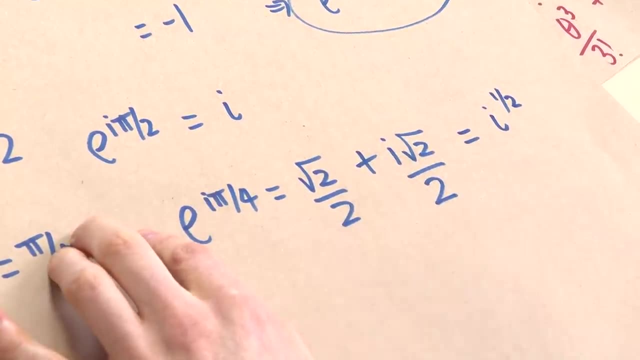 and if you take i to the power of a half, that means multiplying this by a half, which gives you e to the i pi by four. So this is another way of showing the square root of i is given by one plus i, or multiplied by root two over two. 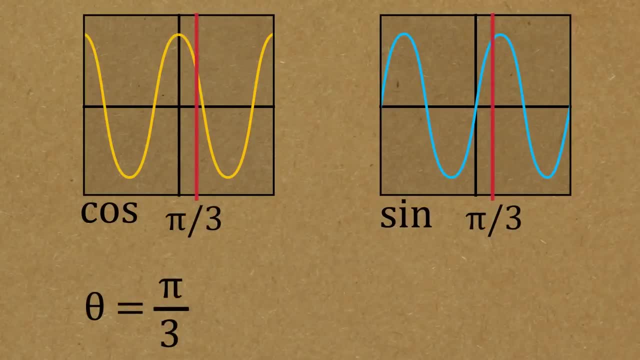 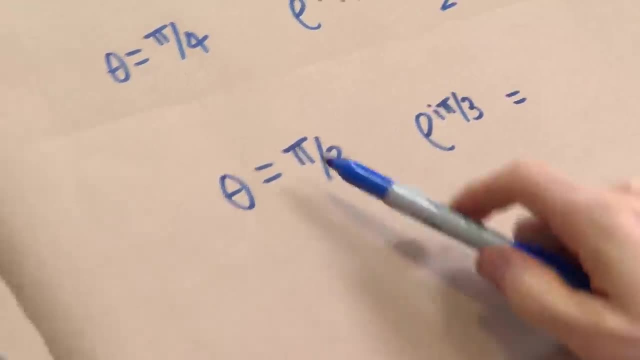 And then the final two that we might want to look at are going to be 60 degrees, So that's pi over three. So e to the i pi over three is going to be cos of 60. So cos of 60 is quite far down. 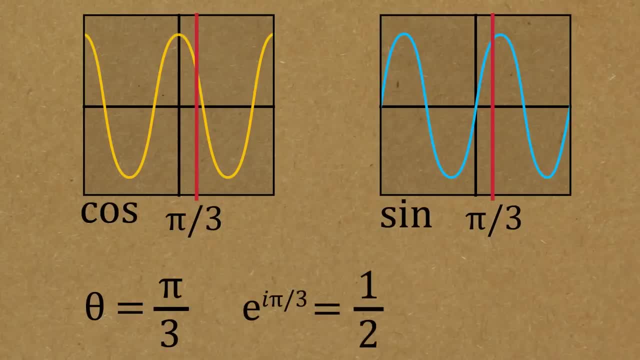 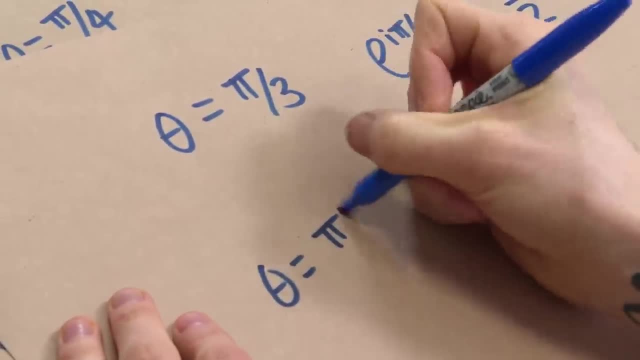 So cos is quite small. So that's a half Plus i times sine of 60.. So that's root three over two, And then the last one, which is my favorite, pi by six or 30 degrees. So I like this one because you bring in a six. 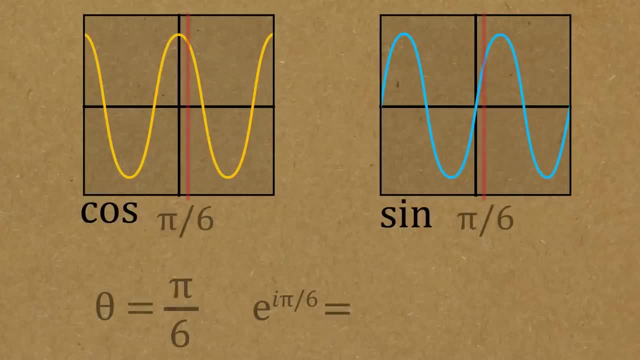 which is a new number we haven't seen in any of our other identities, And that's going to be cos of 30 is root three over two, And then sine of 30 is a half. So we get all of these sort of other identities. 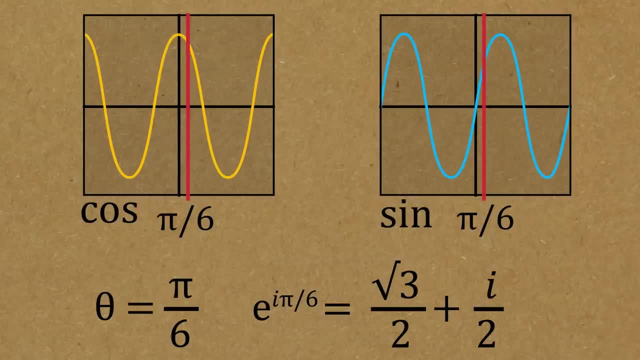 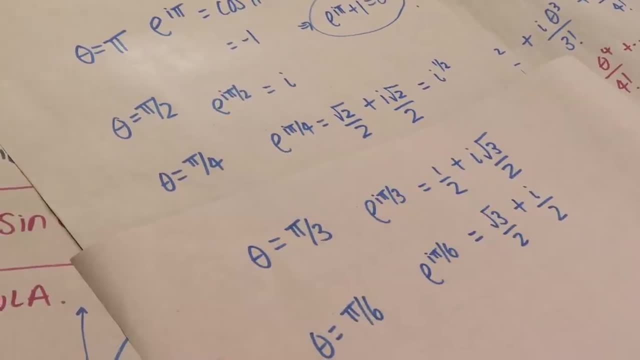 using our most popular numbers from triangles. let's say, You get Euler's identity when it's pi. When it's 90 degrees, you get a definition of i. You get the square root of i when you have 45 degrees. That's quite neat. 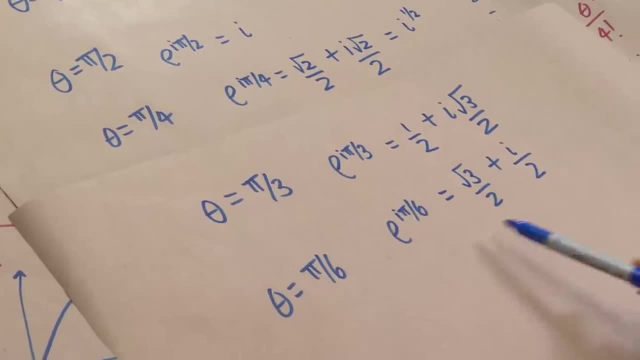 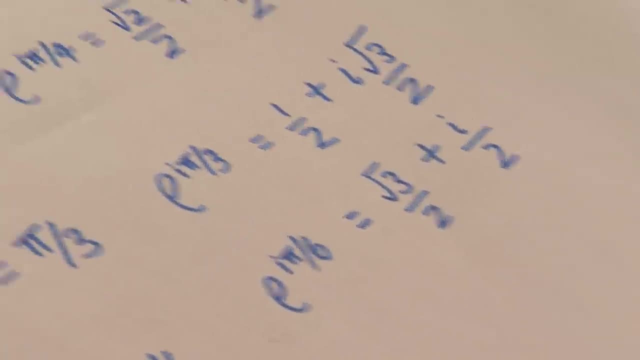 And then we have these two, which I like because you just bring in all of these other numbers. So you have this really cool relationship between six, two, three, i e, All kinds of things. You know what you have to call the sixth one.